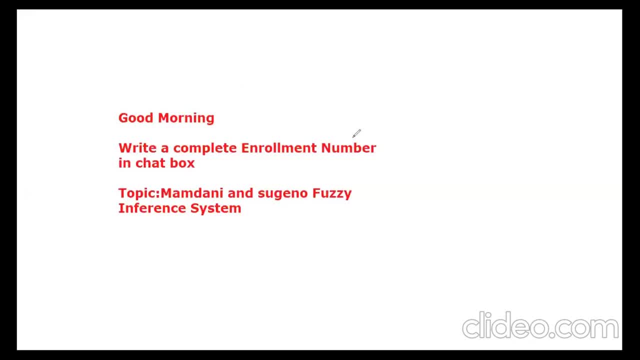 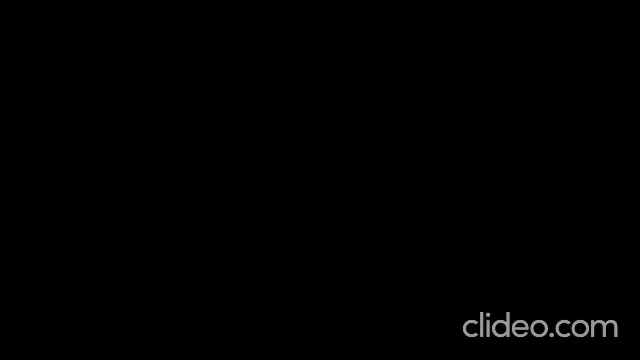 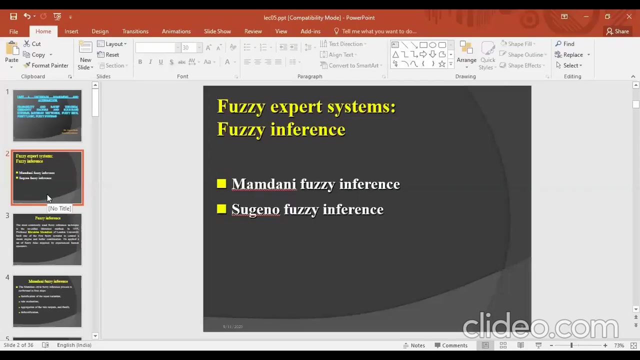 So let's start with the last topic of your unit 1 in section 2, that is, Mamdani and Sugeno inference system. Okay, what is Mamdani and Sugeno inference system? They are the fuzzy expert system, fuzzy inference system. So they are already developed by some expert to solve a 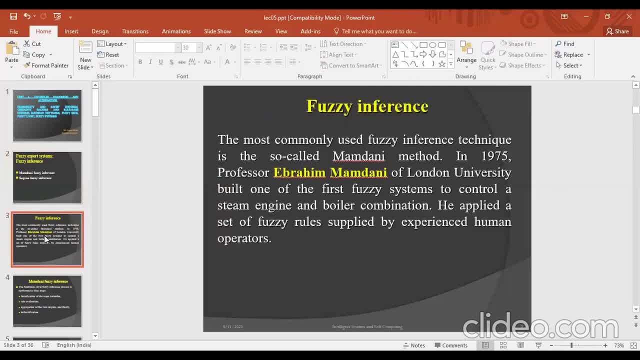 problem using AI. So you can see what is fuzzy inference already. we have covered in previous lecture. The most commonly used fuzzy inference technique is so called as the Mamdani method. In 1974, Professor Mamdani of London University built one of the first fuzzy system to control. 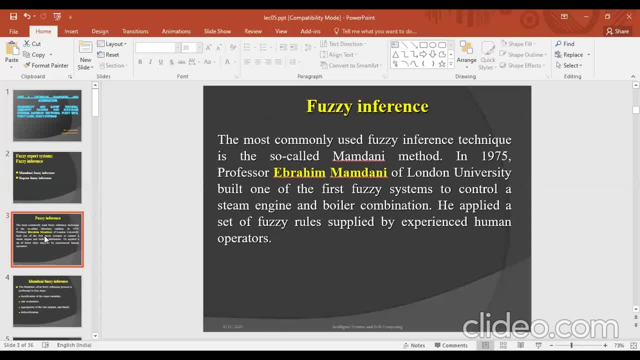 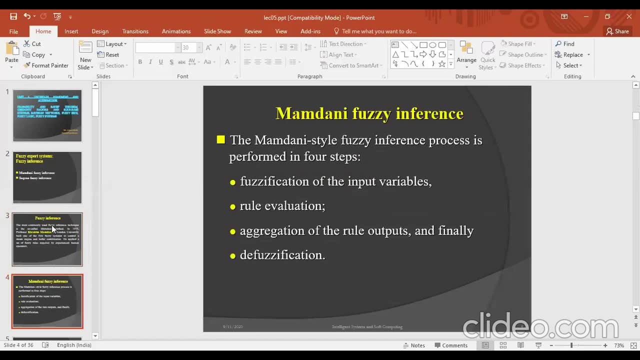 a steam engine And boiler combination. He applied a set of fuzzy rules supplied by experienced human expert. Okay, so in 1975, the Mamdani fuzzy expert system is developed And the Mamdani style fuzzy inference process is performed in four steps. So first step is fuzzification, then rule evaluation, then aggregation of the rule. 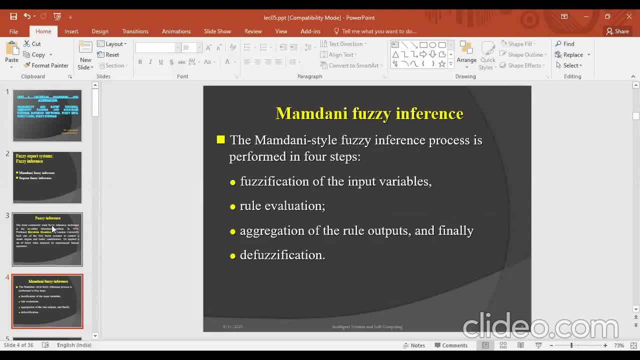 and the defuzzification Already. we know that the fuzzification of the rule and the defuzzification of the rule are different. So we know that the fuzzification of the rule and the defuzzification of the rule are different. We have discussed the previous portion. if we can write if X, then Y is big. So if X is the antecedents. 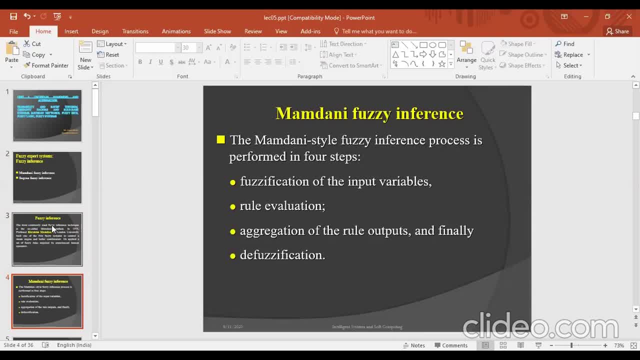 and the Y is B is a precedents. So already we have covered in previous lecture what are the terms that are used, that is, linguistic variables, the variable that have no exact value. that value is called as a linguistic variable, like suppose hot, cold and all Right. So here Mamdani method works for the 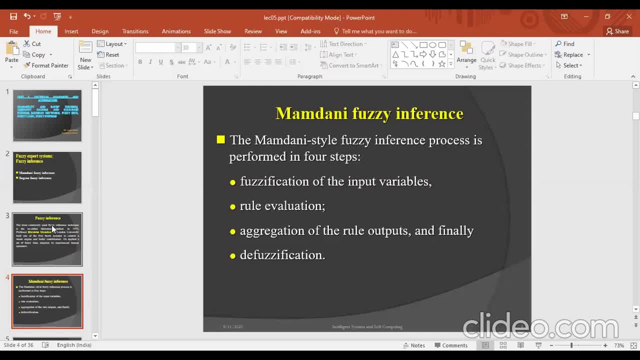 fourth step. The first one is falsification. So why we require falsification? Because the system only understand the CRISPR value. So we have to convert this ambiguous, or the linguistic variable into the value. That process is called as a falsification. 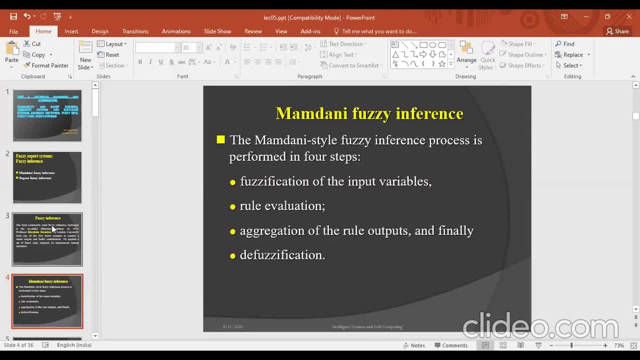 Then rule evaluation. and third one is aggregation of the rule. Sometimes the rule is given: if X is A and Y is B, then Z is C. So we have to evaluate the end operator. So that time we require the aggregation of the rule. And the last step is de-falsification. So what is de-falsification? So only human understand the value of CRISPR value. So the falsification output we have to do is de-falsification. 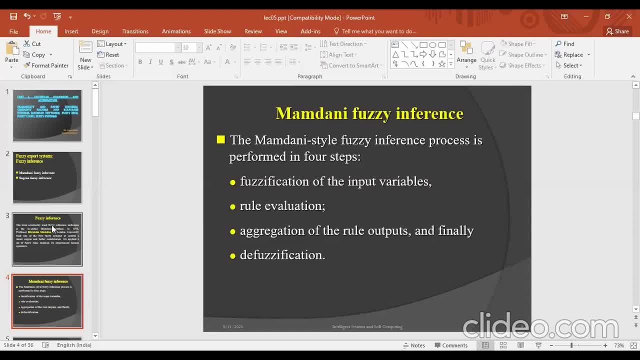 So we have to convert into CRISPR value. That process is called as a de-falsification process. So, one by one, we see how Mamdani Fuzzy Inference System was developed and what purpose we have used Mamdani Fuzzy Inference System. 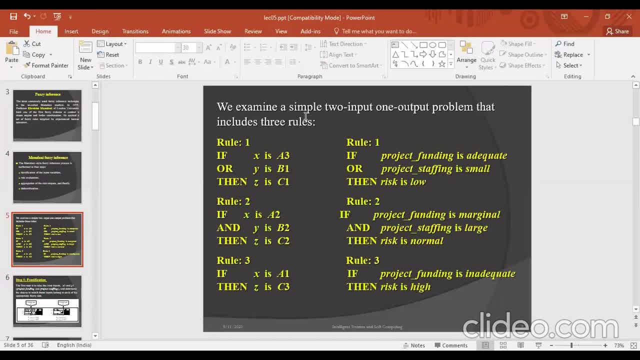 So we take one example: If examine a simple two input and one output problem, that include three rules. The first rule is if X is A3 or Y is B1. Then Z is C1.. So why we require rule? Because system can't have intelligence. We have given the knowledge and based on that knowledge they can take the decision. 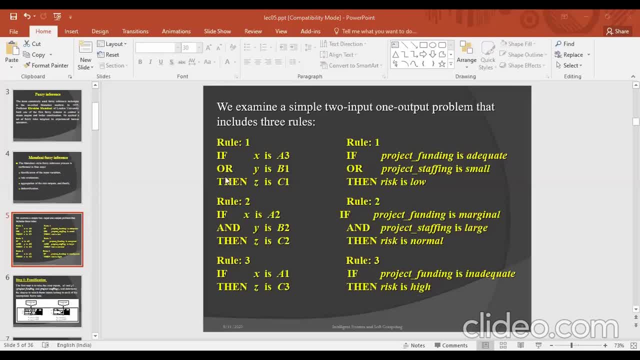 So here we are giving the rules. So, based on the rule, they predict our output. For here I have given the rule: if project funding is adequate or project staffing is small, then risk is low. Okay. The second rule is: if X is A2 and Y is B2, then Z is C2.. Means, if project funding is marginal and project staffing is large, then risk is normal. 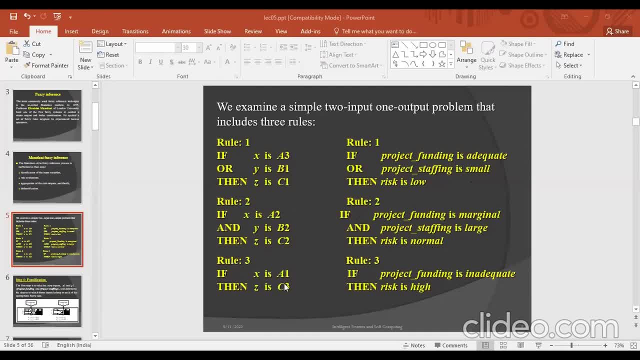 The third rule is: if X is A1, then Z is C3. Then rule number three is: project funding is inadequate, risk is high. Okay, So here I have given the rule and then I have to find our Output of our system. So here, if the, if these are called as the antecedents and these are the precedents or the conclusion of our system, Okay, 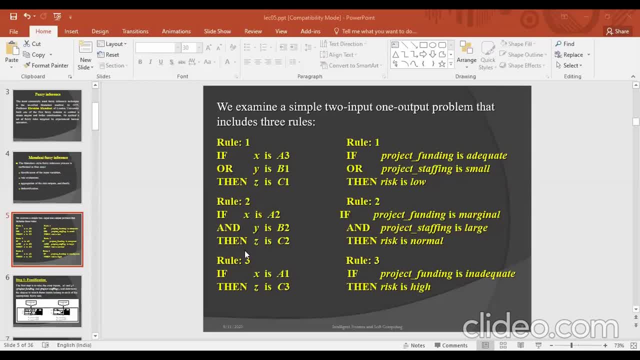 So if X is A2 and Y is B2 is the precedent and Z is C2 is our conclusion. Same as it is here: X is A1 is the antecedent and Z is C3 is our conclusion. Now we check the first. 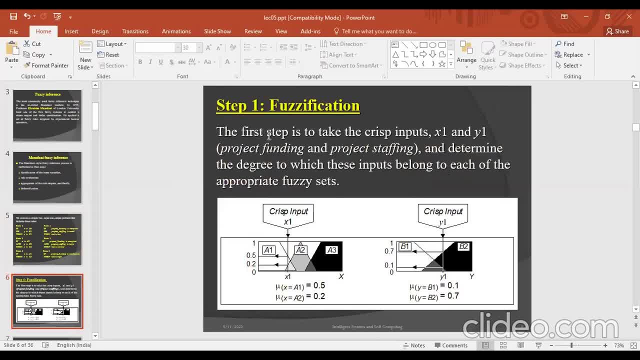 Are our ان آمدین, آمدین, آمدین, آمدین, آمدین, آمدین. here. you can see, i given the value x1, then i converted into a membership function. x is equal. 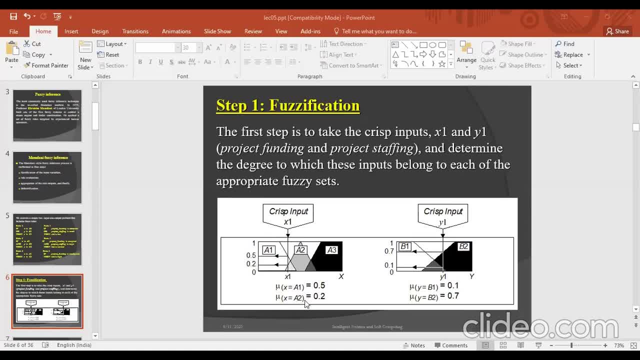 to a1 is equal to 0.5 and x is equal to a2 is equal to 0.2 and y is equal to b1 is equal to 0.1 and y is equal to b2 is 0.7. so mu is your membership function or the membership value. 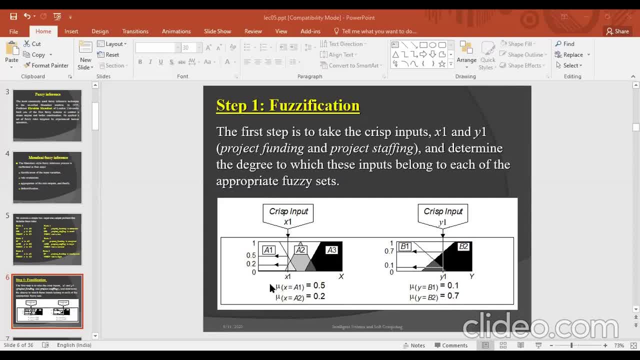 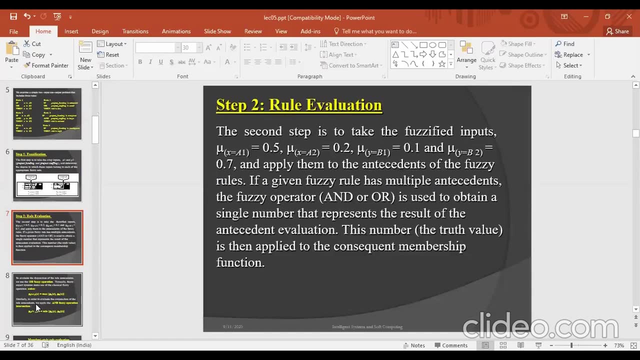 so what is membership value? that represent the involvement of your set in your universal set right. so this is your membership function. that is mu. now the next step is rule evaluation. so we are giving the two rule in our the precedent or first step right. so we have to evaluate this rule because the second step 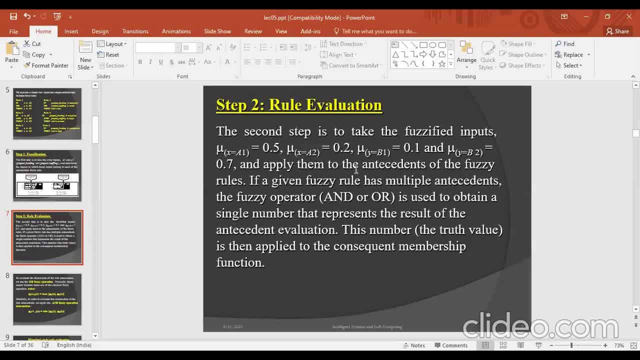 is to take the falsified input then a to the antecedents of the fuzzy rule. If a given fuzzy rule has multiple antecedents, the fuzzy operator AND and OR is used to obtain a single number that represents the result of the antecedents evaluation right. 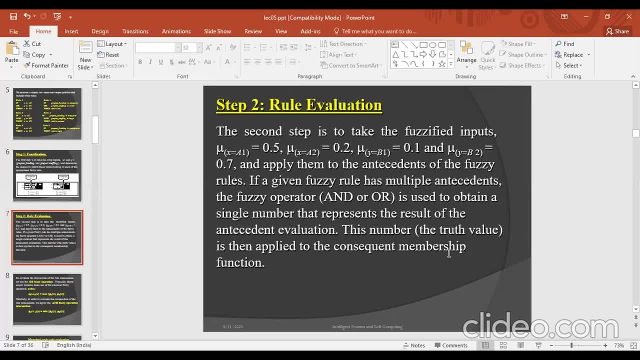 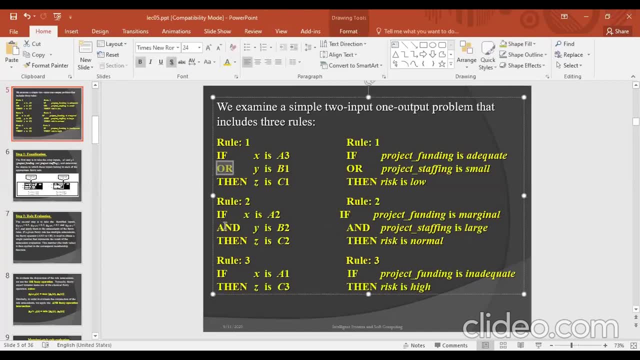 So this number is then applied to the consequent membership function. So in your antecedents part you can see here OR operator is used and the AND operators are used in antecedents. So we have to evaluate this operator in our system right. 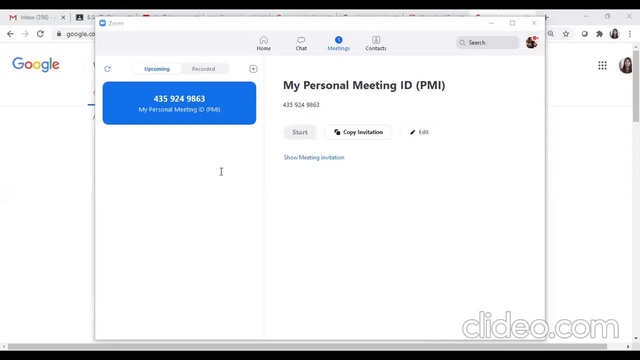 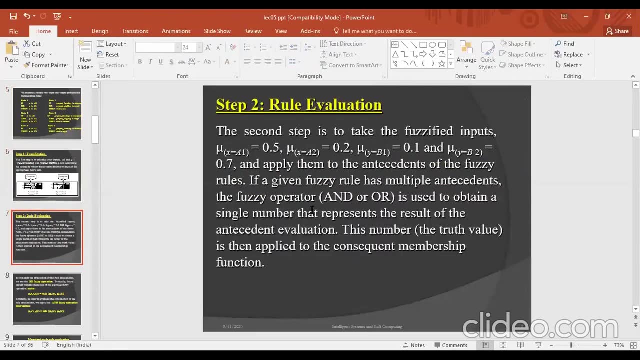 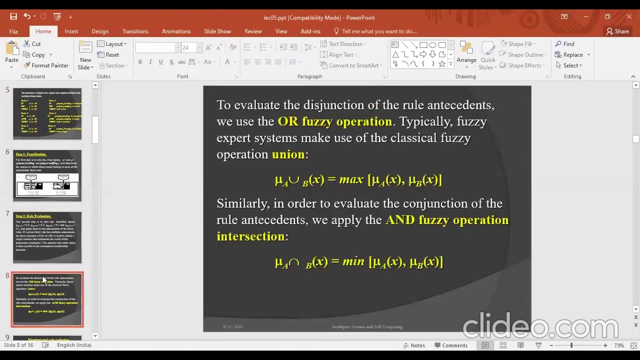 So first of all, first we are converting the input value into a fuzzy value and then the second step is the rule evaluation. So we have to solve this operator AND and OR right To evaluate the destruction of the rule, the antecedent, we use the OR- fuzzy operation. 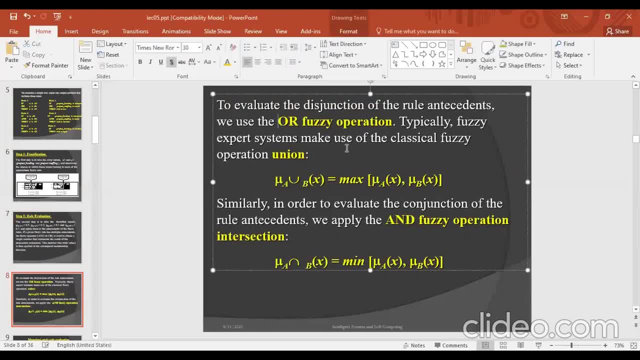 So what you have to do, If you have given the OR operator, then you have to find the value of the operator AND and OR. So you have to find the maximum value of your given two inputs Here: the membership value of fuzzy set A and the membership value of fuzzy set B. 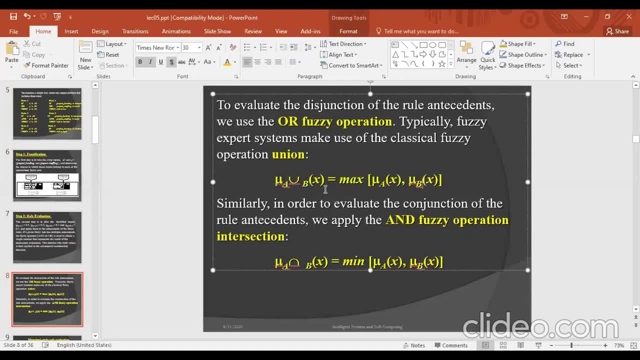 Then what is the union operator? So mu of A, union B is equal to maximum of union of A in comma. membership value of fuzzy set B, So same as it is for AND operator. you have to find the minimum value of two given input set right. 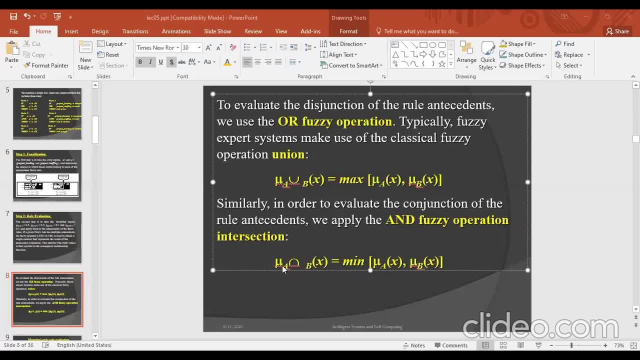 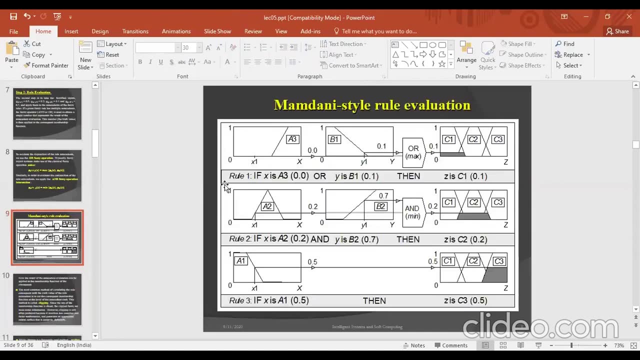 So you can find the. You can find the intersection of two set of fuzzy set. okay, Now the next step is: So first step is falsification, then rule evaluation, then third step. you can see here in graph format: 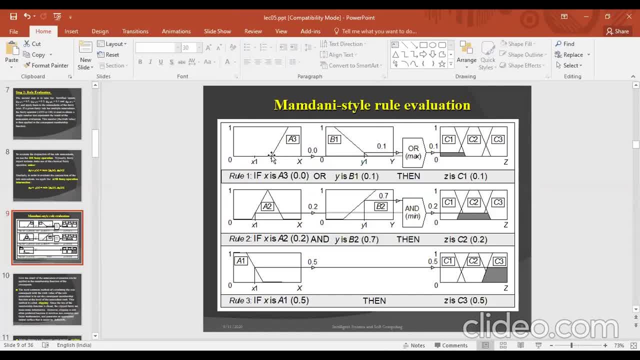 So if X is A3,- that is your rule- that the value is 0 and Y is B1,, that membership value is 0.1, then you have to find here is the OR operator is used right. So you have to find the evaluation of the two antecedent. 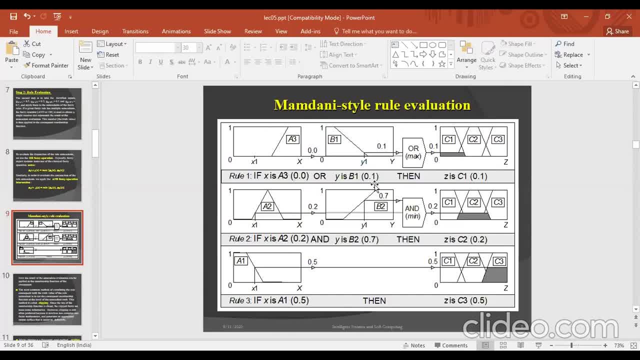 that is the maximum of 0, 0.1.. So 0.1 is the maximum value of your system right, Same as it is in AND operator. we find the minimum value of your given two set Here. if X is A2, their value is 0.2. 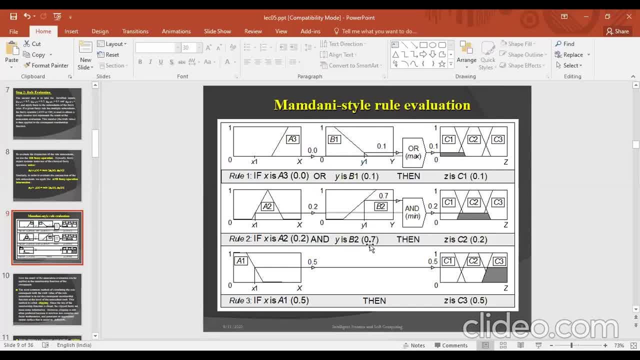 and the Y is B2,. their value is 0.7.. Then what is the output of your Z? So Z is C2, that is minimum of A2, B2, means 0.2, 0.7.. 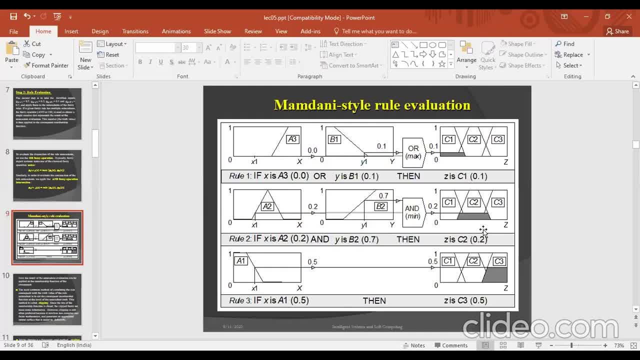 So minimum value is 0.2.. Here that represented in here graph: okay, Same as it is. if X is A1, then Z is C3. So directly, A1 value is transferred to the C3. So 0.5,, then 0.5, okay. 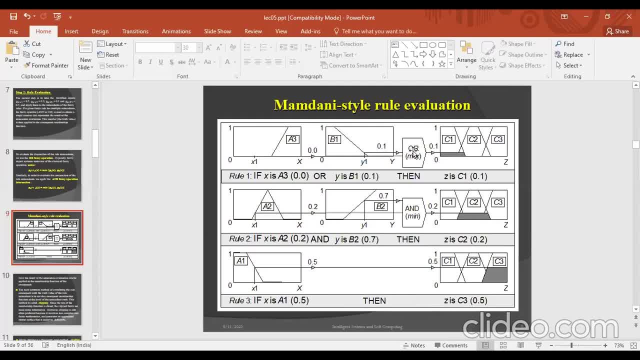 Clear All the students. So what is AND operator and OR operator? So in AND operator you have to find the minimum of given two input and in maximum OR operator you have to find the maximum value of given two input. Okay, 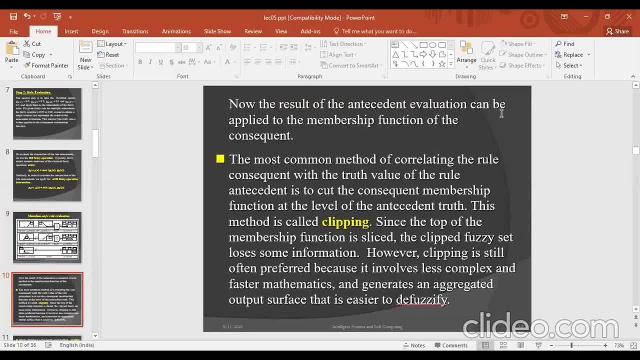 Now the result of the antecedents evaluation can be applied to the membership function of the consequent. The most common method of correcting the rule consequent with the truth value of the rule antecedents is to cut the consequent membership function at the level of antecedents' truth. 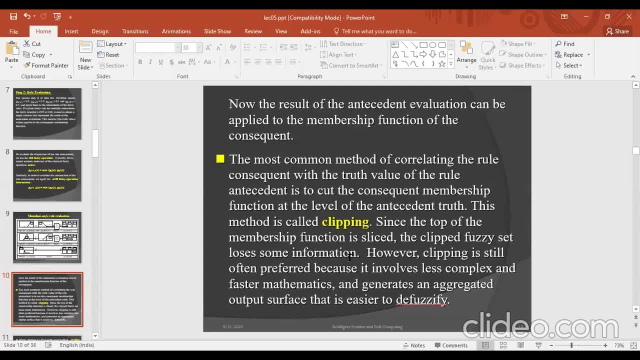 This method is called clipping. Since the top of the membership function is sliced, the clip possesses low-sum information. However, clipping is still often preferred because it involves less complex and faster mathematics and generates an aggregated output surface that is easier to disfazify. 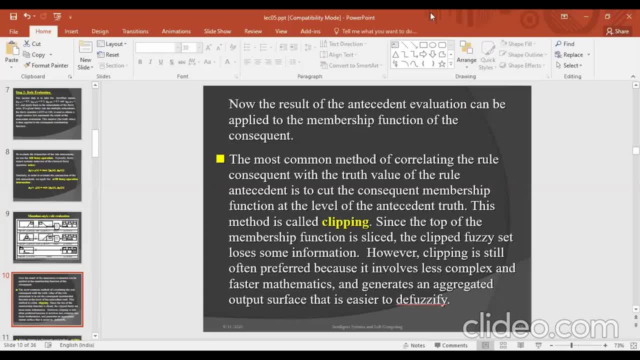 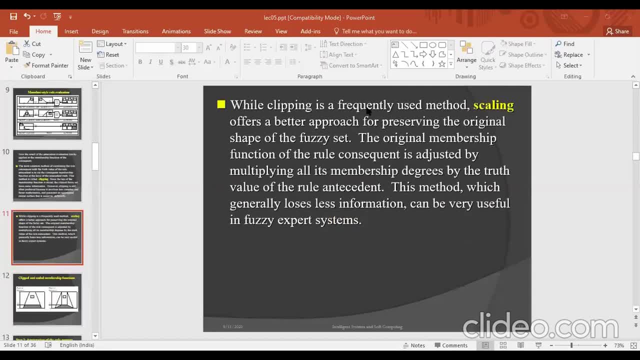 So what is clipping? I show you with examples So you can see that in this example. so you have clear what is clipping method. You can see here in graph format why clipping is a frequently used method and scaling offers a better approach. 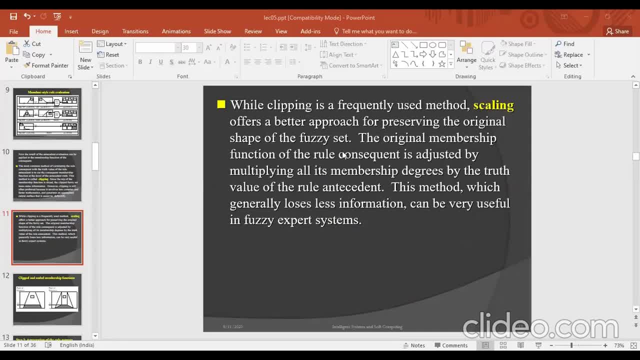 for preserving the original shape of the fuzzy set. So here the clipping method is used to preserving the original shape of the fuzzy set. The original membership function of the rule consequent is adjusted by multiplying all the numbers. This method has all the membership degree. 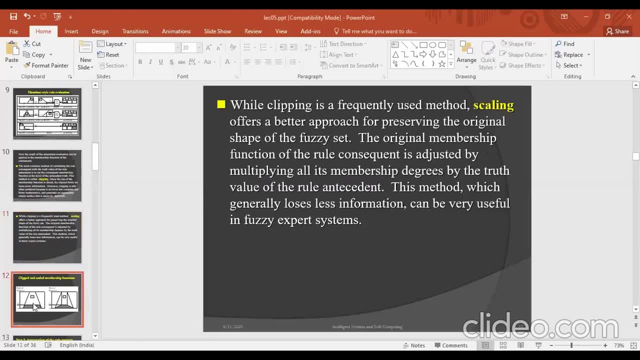 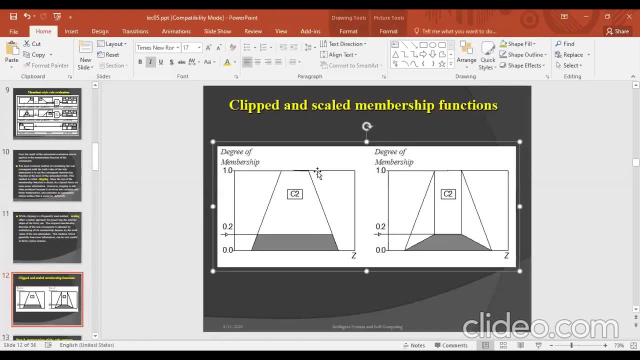 by truth. value of the rule. antecedents. You can see here in graph format: you are fuzzify and you are aggregate the output Right. So this is your left side, is your output of your fuzzy set. And then you are converting the clipping method. 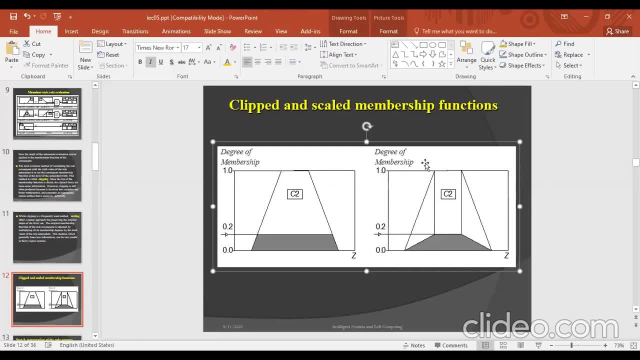 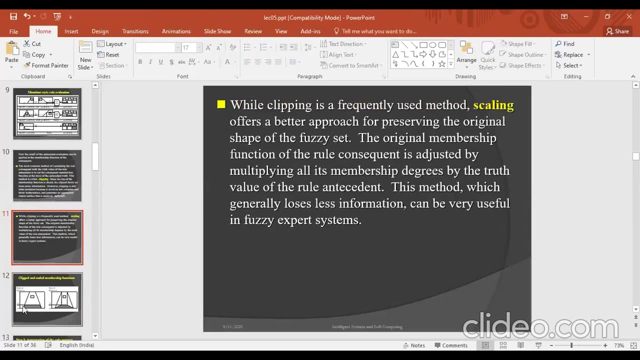 That is your scaled output. So here, the right hand side, is the output of your clip and the scale multiple function Why we are using this method. Thank you for converting scaling or for a better approach for preserving the original shape of fuzzy set. 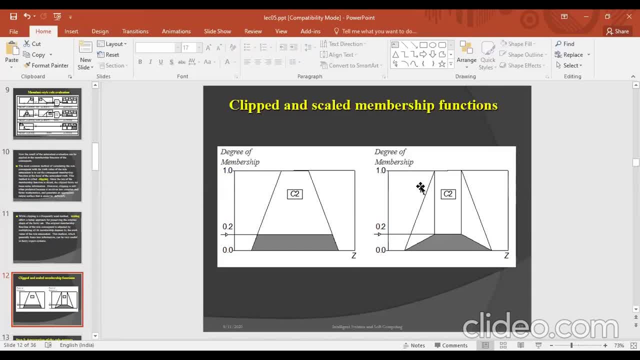 So that's why we are converting this, our input, into clip method or the fuzzy set. Okay, you can see, the left hand side is the degree of membership and the crisp, your fuzzified output, and you are scale in this manner. Okay, so this is your clipping or the scaling method, because we are converting into scale method so we can't lose our original data. 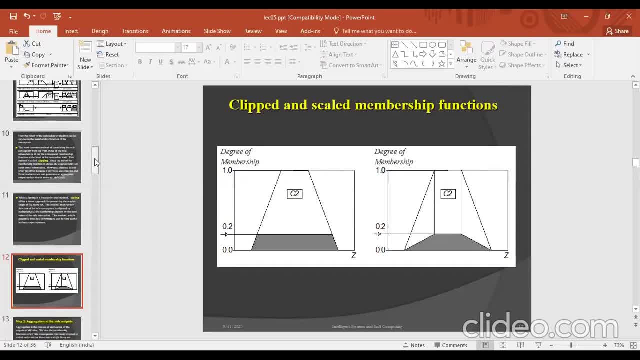 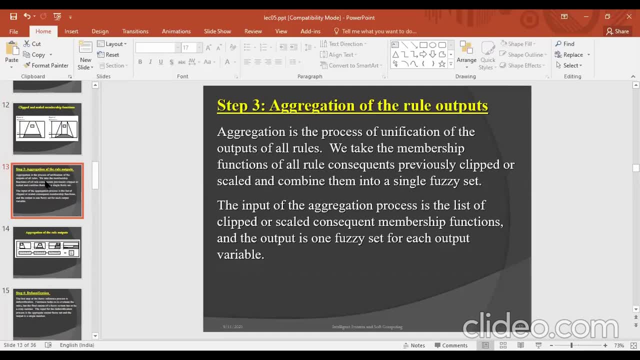 So that's why we are clip the data or scale the data. Okay, now the third step, that is aggregation of the rule. So what is aggregation? So you have given a two antecedents, then you have to compulsory give the output of two aggregation, right? 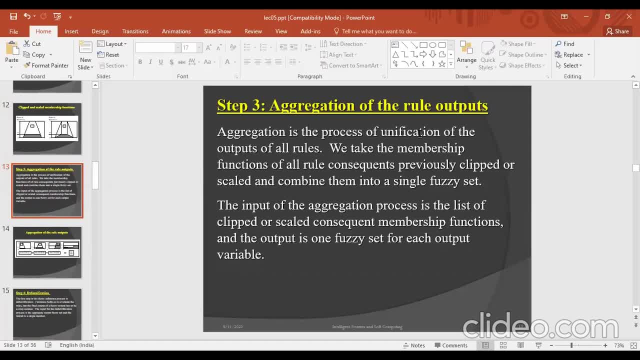 So aggregation is the rule. It is the process of unification of the output of all the rule. So we take the membership function of all rule consequent previously clip or scale and combine them into a single fuzzy set. So the input of the aggregation process is the list of clip or the scale consequent membership function and the output is one fuzzy set for each output variable. 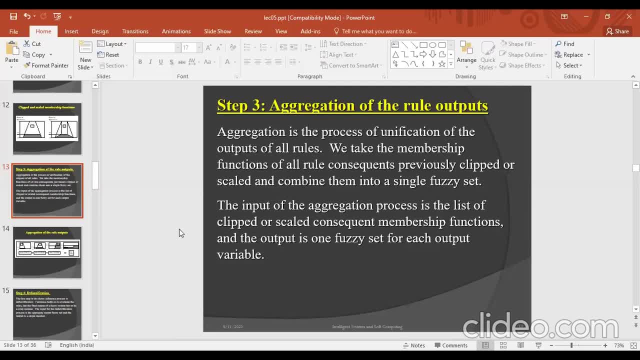 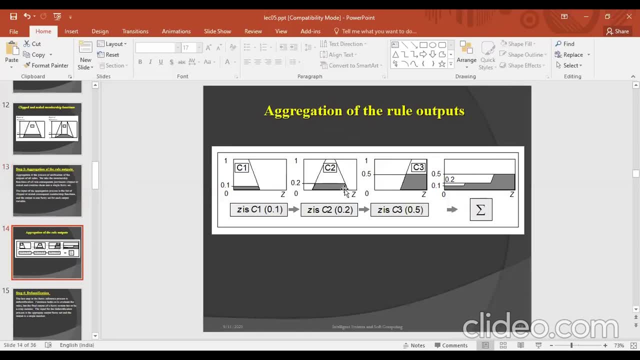 So you have to aggregate all the input antecedents. So let's conclude the value of final unique value. that is called as the aggregation. So you can see in this example, So you have clear: if you have given Z is C1, that value is 0.1 membership value, then Z is C2, that value is 0.2.. 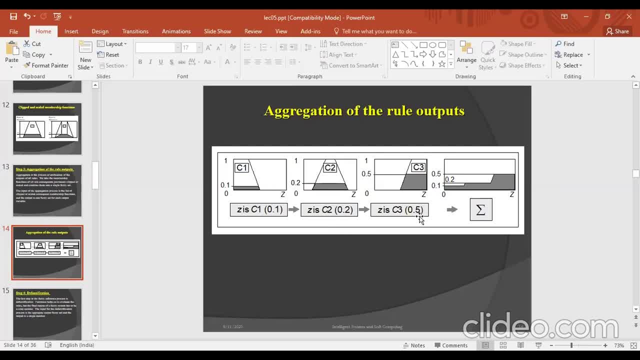 Then you have to aggregate this value. Z is, if Z is C3, 0.5.. Now you have to aggregate this. all the rules output That 0.1, 0.2 and 0.5.. So here you can see the aggregation of the given input, that is, C1, C2 and C3.. 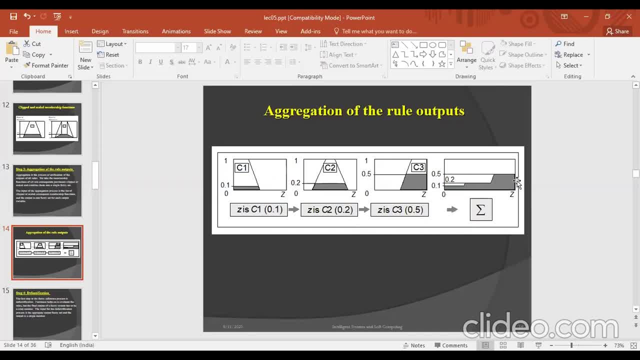 Here 0.1, then 0.2 and 0.5.. So aggregation is the required for your conclude, the final output of your fuzzy set. Okay, So you have given Z is C1, Z is C2 and Z is C3.. 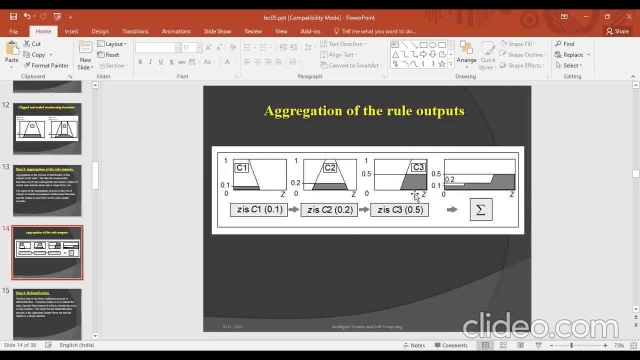 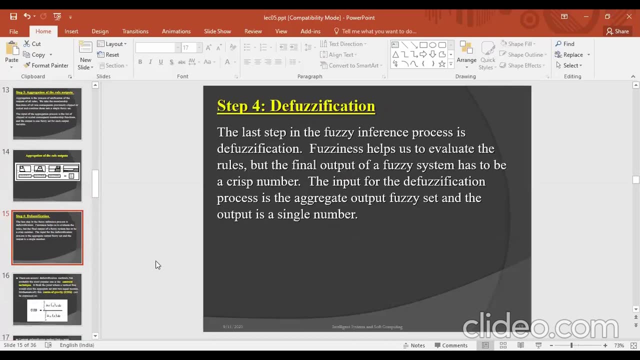 Then you have to aggregate of the rule output. So here aggregate, Here aggregate output. you can see in the last graph. Okay, Now the last step of your Mamdani method is the defuzzification. So what is defuzzification? The last step in fuzzy inference process is defuzzification. 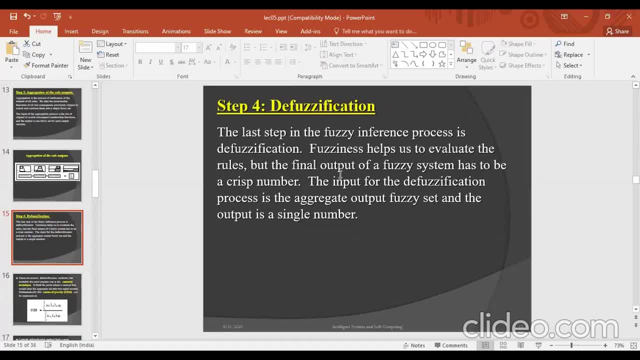 Fuzziness help us to evaluate the rule, But the final output of fuzzy system has to be crisp number. The input for the defuzzification Process is aggregate output, fuzzy set and the output is a single number. Now you have to give the output of your fuzzy system. 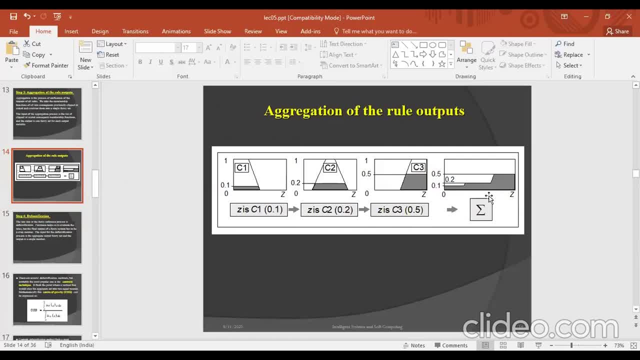 So only system understand or the user understand the crisp value. Suppose you are giving the output of this graph means aggregation of the rule output, Then system can't understand the decision of your system. But we have to convert this fuzzy output into crisp value. 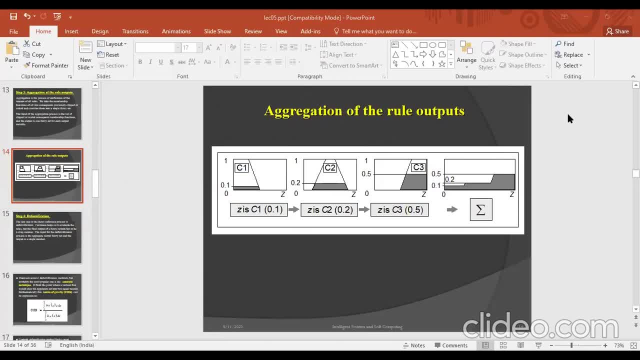 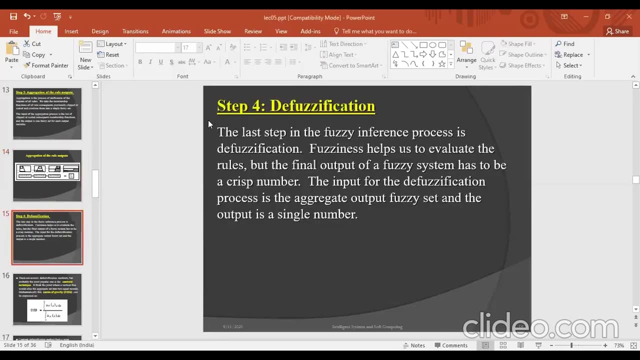 This process is called as a defuzzification. Okay, Here in defuzzification, you give the input as the aggregation of the rule output And convert it into the crisp value. So these are the four steps that follow by Mamdani method. 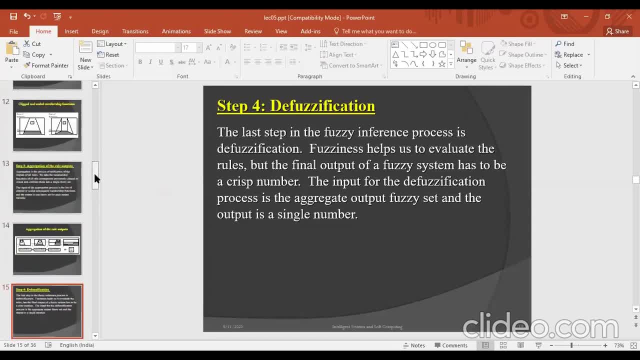 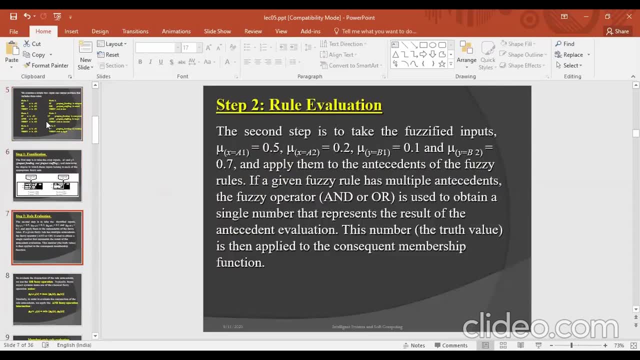 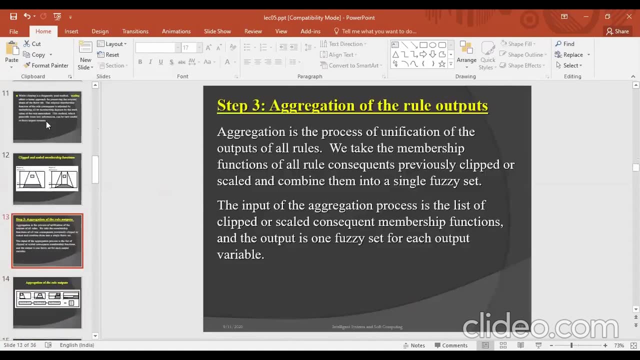 The first one is Fuzzification. Then you have to solve the operator means. you have to convert into rule evaluation. The second step is rule evaluation. The third step is clip and the scale, membership function or aggregation of the rule output. And the last step is defuzzification. 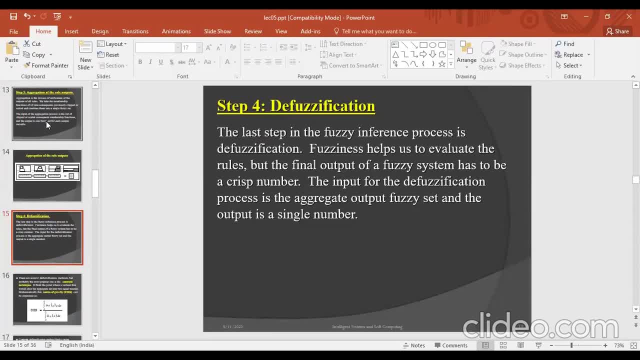 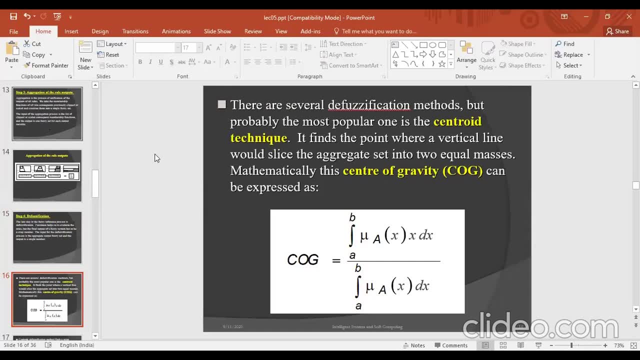 So these are the four steps that Mamdani method follow. And what is the defuzzification method mostly used in Mamdani? So there are the several defuzzification method, But the probably the most popular one is the centroid technique. So it find the point where a vertical line would slice the aggregate set into two equal message. 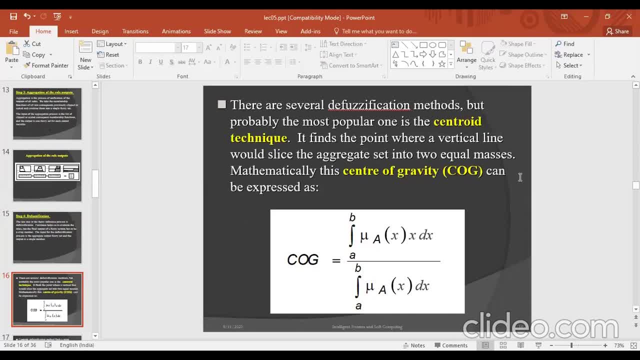 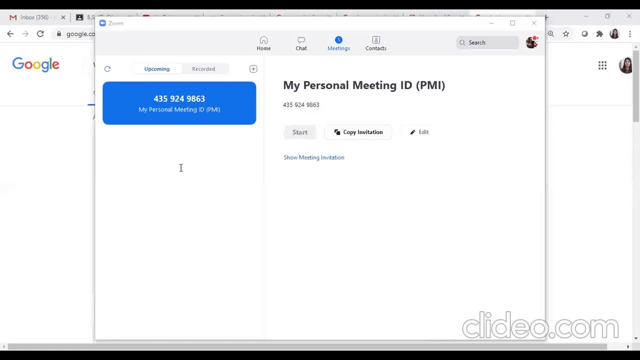 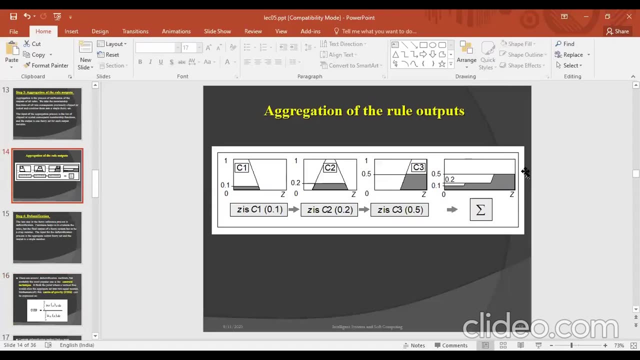 Okay, Mathematically this is the center of gravity. Now you have conclude this output. that is your aggregation of the all the rule. But now you have to give the input value. Here you can see: the output of aggregation is this graph. Now you have to find the any crisp value from given this area. 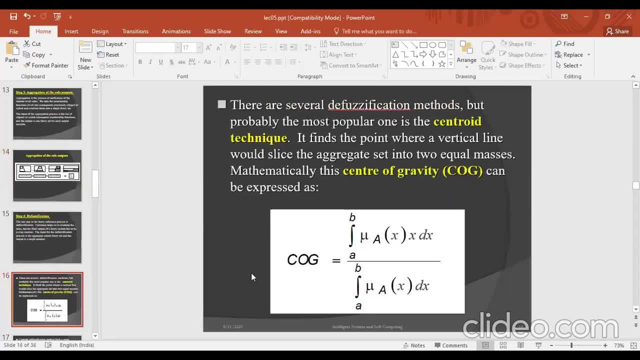 So, using center of gravity, This rule is: this formula is used to calculate the crisp value from your given fuzzy set. The center of gravity is equal to integration of A to B. The membership value of set X into multiplication into X into DX, Divided by integration of A to B. membership value of set X into DX. 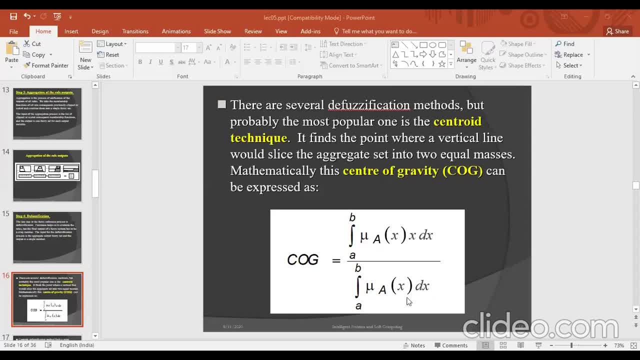 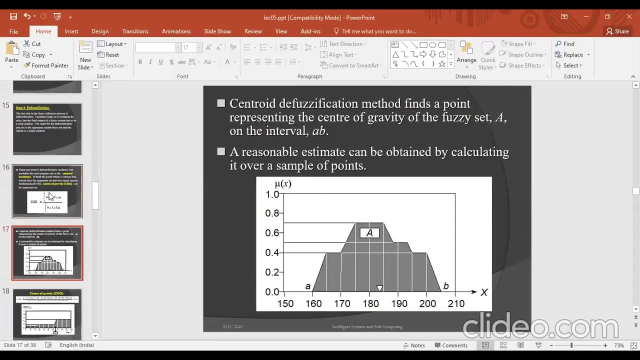 Okay, This is the formula for finding the center of gravity and find the unique value or the crisp value from your given fuzzy set, Because at last, the user can understand only crisp value, So we require fuzzification. Now you can see the calculation of center of gravity. 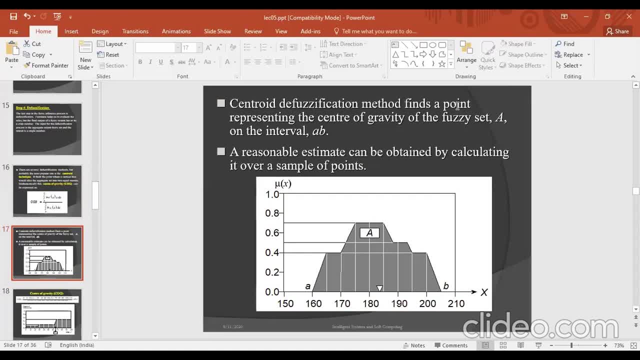 So centroid defuzzification method: Find a point representing the center of gravity of fuzzy, set A on the interval A- B. A reasonable estimate can be obtained by calculating it over a sample of point. Suppose you have given in X axis the value of input X and the converted that into crisp membership value, that is mu of X. 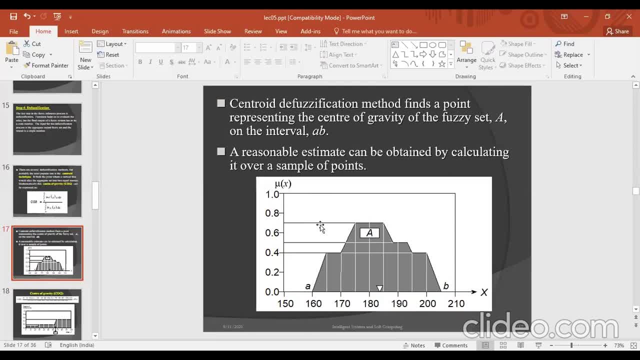 Now we reach to our final conclusion, that is, rule evaluation And aggregation of your given input. Then we have to find the unique or the crisp value. So here we have to find the unique value that belong to our output set. So how you can calculate using center of gravity method. 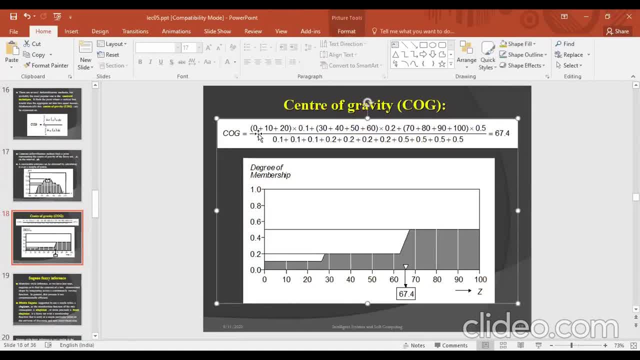 Here you can see example: COG is equal to 0 plus 10 plus 20 into 0.1.. What is the value of this input? that is 0,, 10, 20.. The value input is 0.1.. 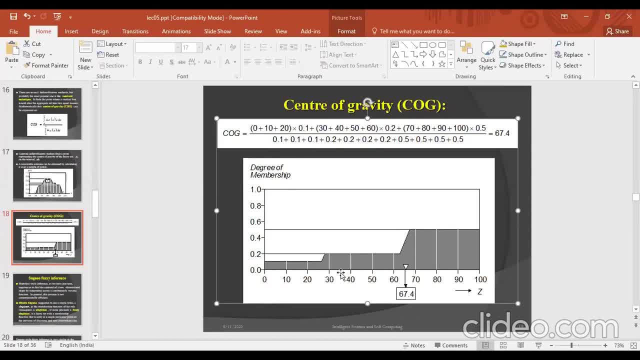 So multiply 0.1.. Plus 30,, 40,, 50 and 60 into multiplication 0.2.. Now 70,, 80,, 90 and 100, their value 0.5.. Right So now and below, divided by the base value of your set, that is 0.1, 0.1 and 0.1. 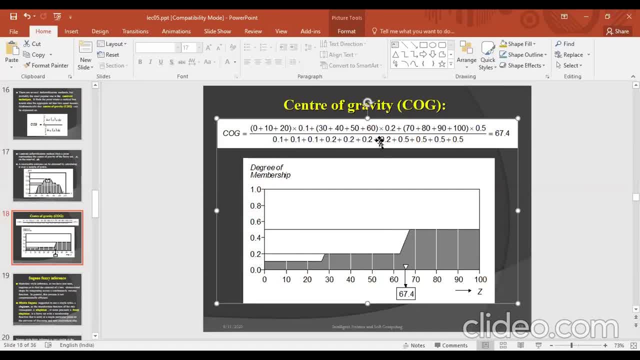 And for 30,, 40,, 50 and 60 their value is 0.2.. And for 70,, 80,, 90 and 100 their value is 0.5.. So I get the output 67.4.. 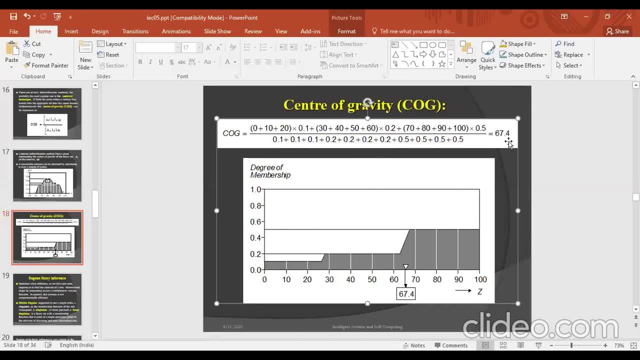 This is your center of gravity of your output. Okay, This is your Mamdani method. Anyone who have not understand any step, then you can tell me. I again repeat this theory. Otherwise we start the Sugeno method. Here you can see the center of gravity. 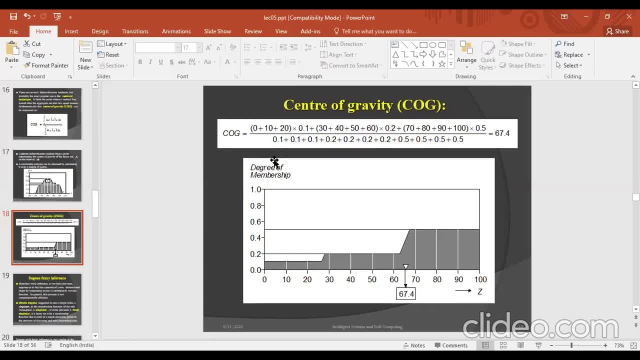 Here you can see the center of gravity. If you have question, then you can ask me in the chat box. Yeah, You can write your question in chat box. If you not understand any step of the Mamdani method, then you can ask me in the chat box. 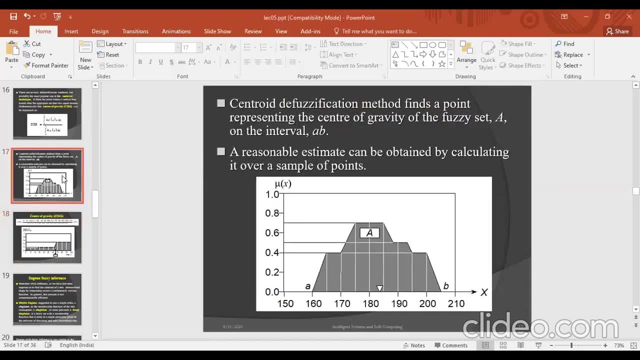 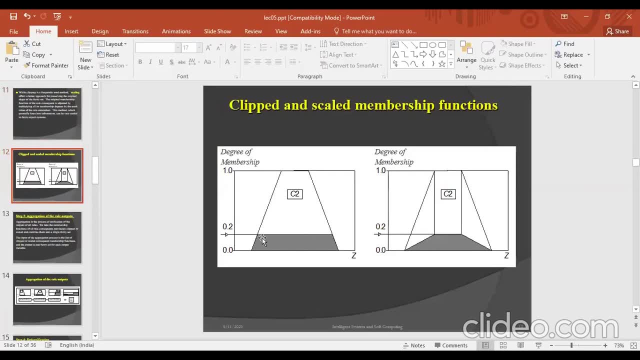 What is clipping, So why we are using clipping. Once again, I repeat So you can see here this is my output of rule, But sometimes the data may be lost. Suppose we are evaluate the two rule of the antecedents, Then sometimes the data. 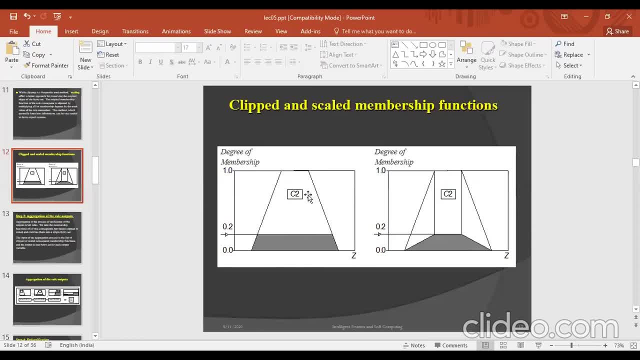 So I convert the crisp value into fuzzy set Right. So sometimes it, sometimes maybe it lost the data. So that's why we are clip or the scale data, So we can't lose our important data. For that purpose we are scale or the clip. 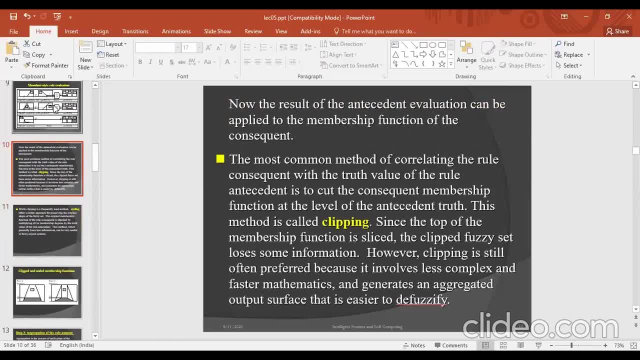 You can see here Now the result of the antecedents evaluation can be applied to the membership function of the consequent. The most common method of correcting the rule consequent with the truth value of the rule Antecedents is to cut the consequent membership function at the level of antecedents truth. 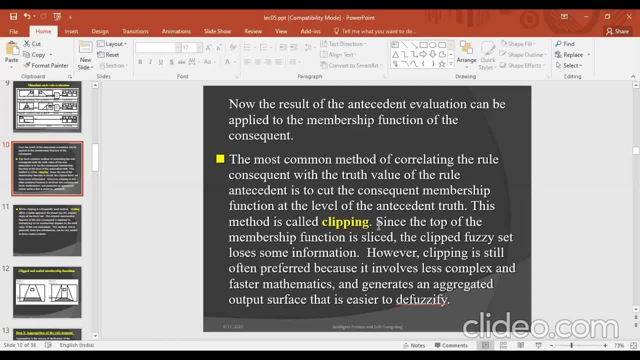 So this method is called as a clipping. Since the top of the membership function is sliced, The clip fuzzes at losses some information. To prevent the loss of your function, we are using clipping. However, clipping is still often preferred Because it involves a less complex and faster mathematics. 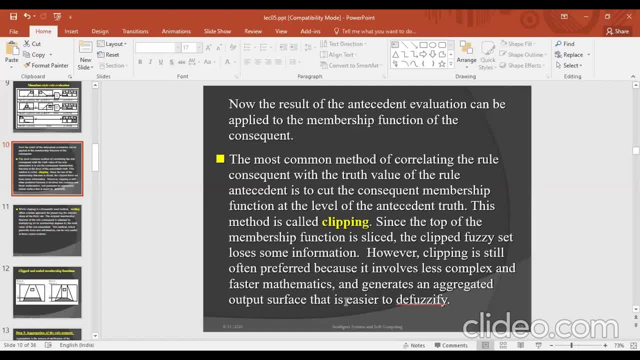 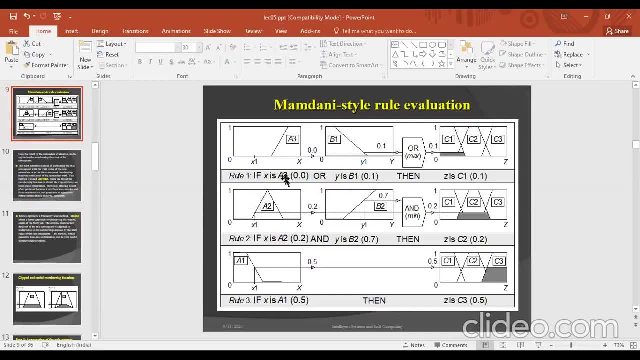 And generate an aggregated output surface That is easier to defuzzify. Okay, So you are in rule evaluation. You are converting this fuzzy value And evaluate this antecedents part of your rule, But sometimes there may be chance to cut your original data. 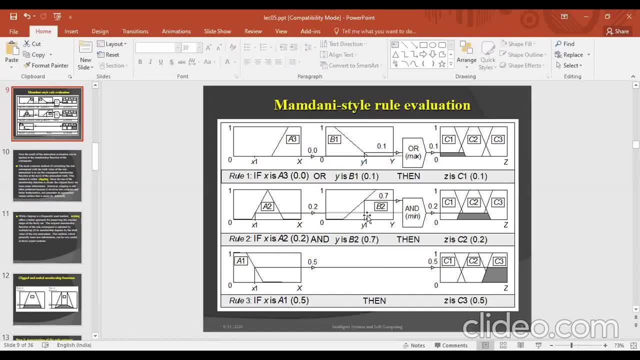 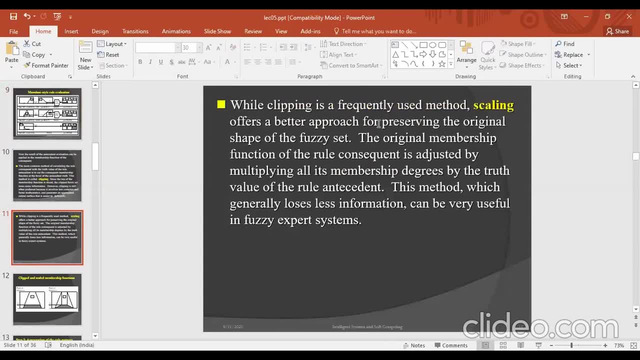 Because when you are converting your crisp data into fuzzy set, Sometimes maybe the meaningful information may be lower, But the clip or scaling is used for the better approach for preventing the original shape of your fuzzy set. Okay, So the original membership function of the rule consequent is adjusted by multiplication. 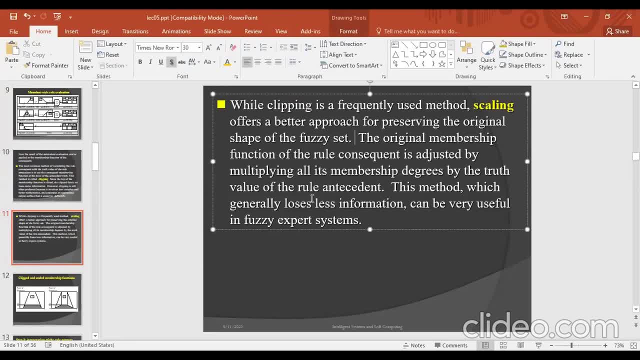 By multiplying all its membership degree by the truth value of the rule antecedents. So this method, which generally losses less information, can be very useful in fuzzy expert system, Because if you are developing a medical diagnosis system And sometimes you are lost the meaningful information from your given data. 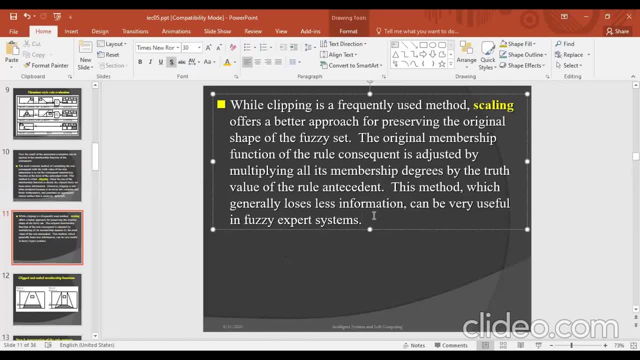 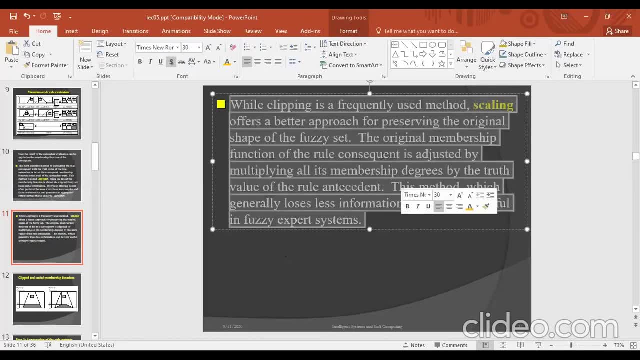 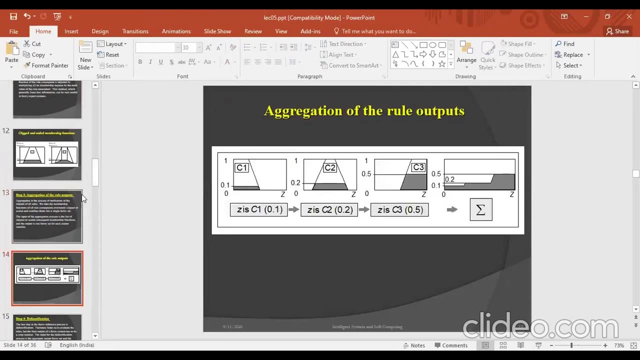 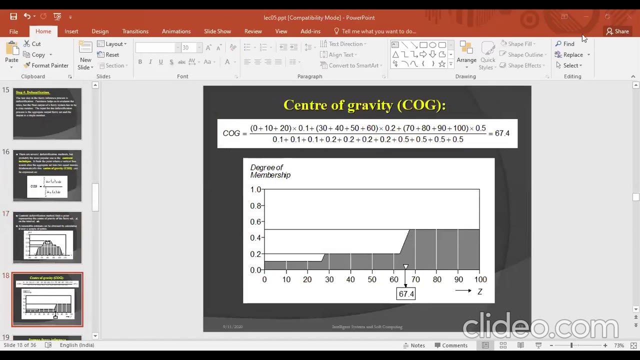 Then it is very dangerous to patient diagnosis a disease. Okay, So next time we require this process- scaling and clipping. Okay Clear, Are you satisfied with my answer? Anyone have a question? Then you can ask me a question, Then we can convert. 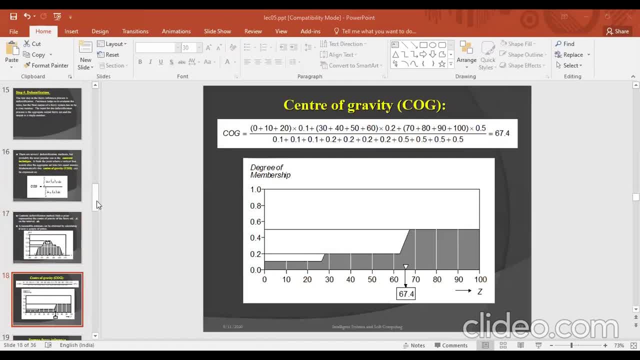 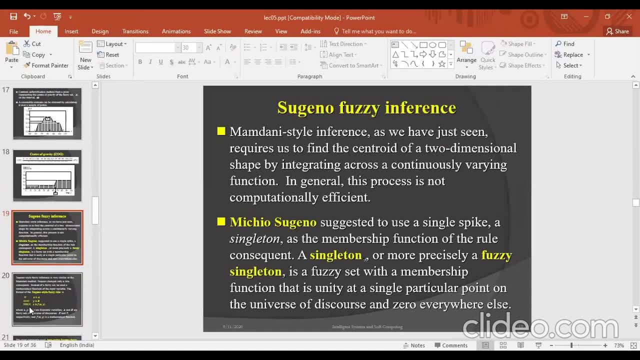 We are go to the next, That is Sugeno method. So this system are already developed by fuzzy expert. That Mamdani and Sugeno, So Mamdani style. Now we start the Sugeno fuzzy inference, So Mamdani style inference, as we have just seen. 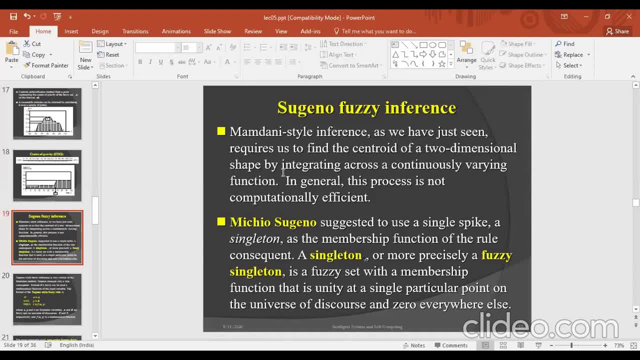 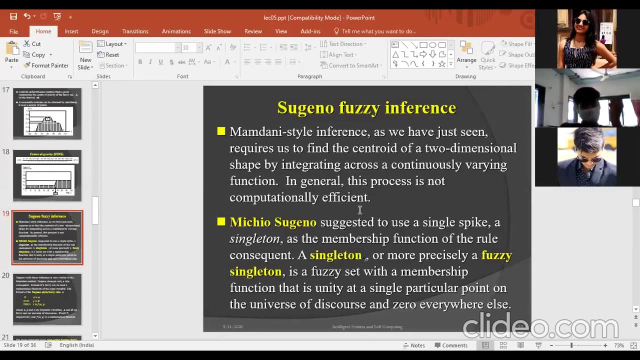 Require us to find the centroid of two dimensional set by integrating across a continuously varying function. In general, this process is not computationally efficient. Now we have to find what is Sugeno method and where we use Sugeno method. So what are the advantages over the Mamdani method? 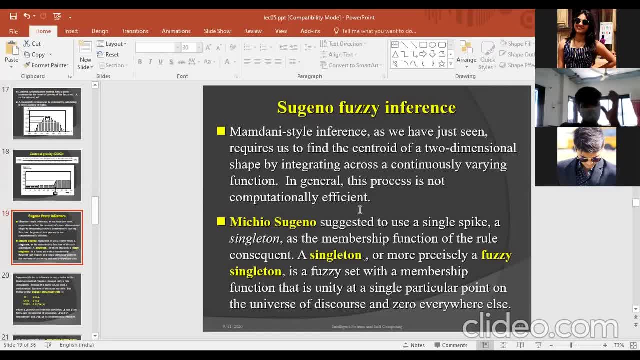 In Mamdani method we have find the two dimensional set of integrating across a continuous varying function, But Sugeno. Sugeno suggested to use a single spike or single tone. Here you can. I show you one example So you have clear why we use Sugeno. 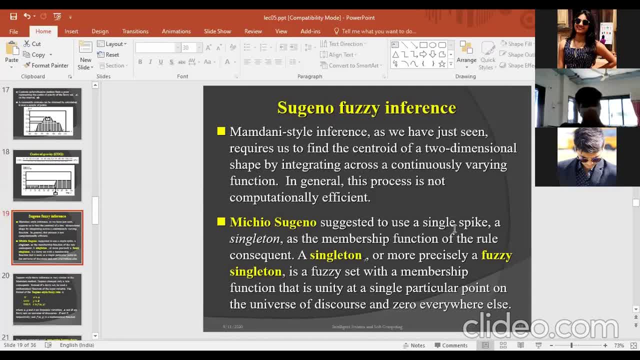 So Sugeno. Sugeno suggested to use a single spike or single tone as the membership function of the rule consequent: A single tone, or more precisely a fuzzy single tone is a fuzzy set with a membership function That is unity at a single particular point on the universe of this closure and zero everywhere else. 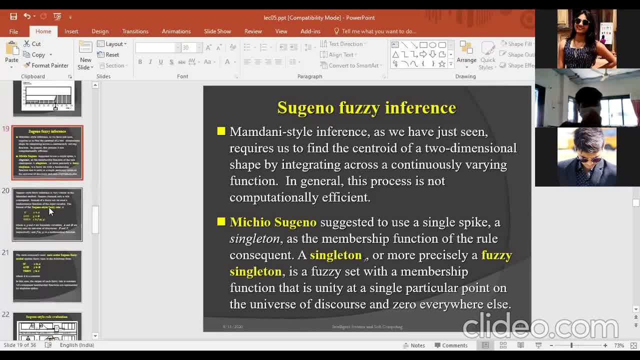 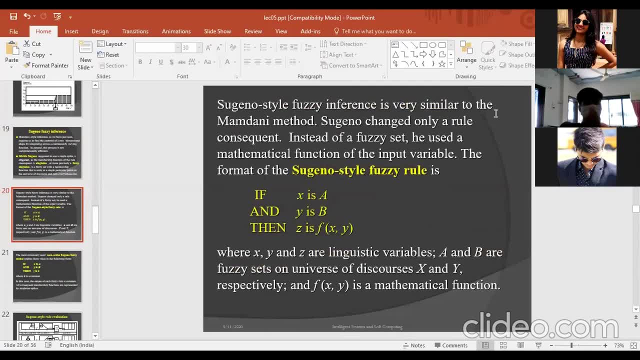 You can see. I give one example So you have clear where we use Sugeno method. So Sugeno style fuzzy inference is very similar to Mamdani method, But Sugeno changed only rule consequent. Instead of fuzzy set he used a mathematical function of the input variable. 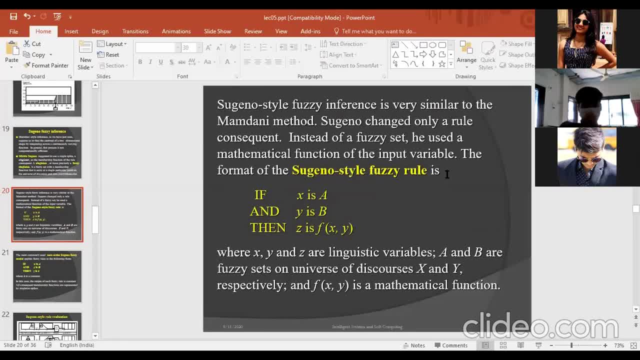 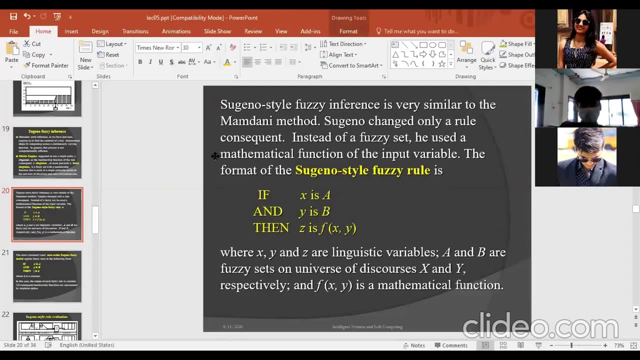 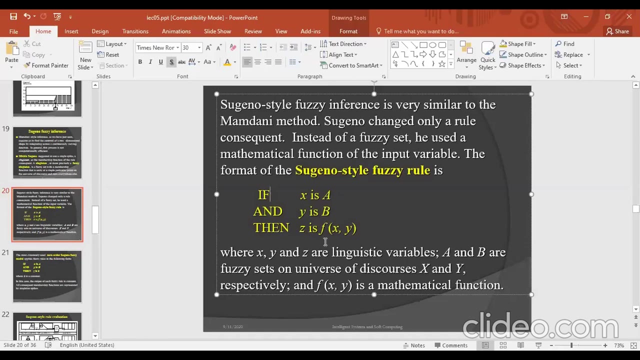 The format of the Sugeno style fuzzy rule is here. You can see, in Mamdani method we are converting our crisp data into membership function, But in Sugeno method we are using the mathematical function. If your rule, if x is a and y is b, then z is f of x comma y. 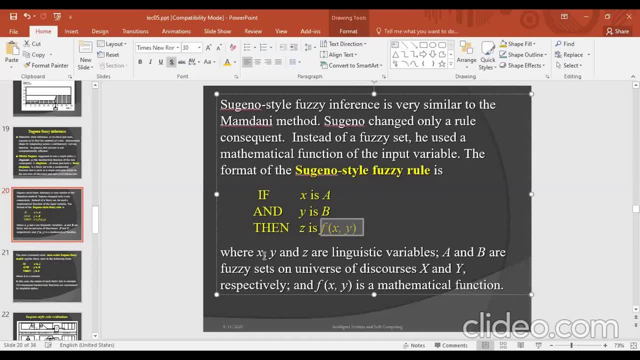 So we are using here mathematical function Where x, y and z are the linguistic variable. Already you know what is linguistic variable: The variable which have not exact value. Sometimes you can use cold hot. speed is fast, slow. This type of value variable is called as a linguistic variable. 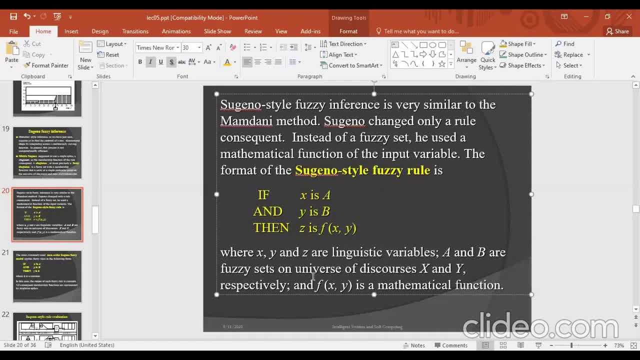 Then a and b are the fuzzy set on the universe of this closure, x and y respectively, And f of x, y is a mathematical function. So Sugeno has development system that has the output is a mathematical function: z, x, comma, y. That changed in the Mamdani method. 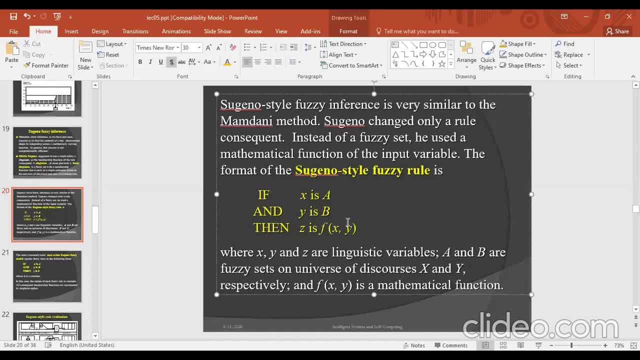 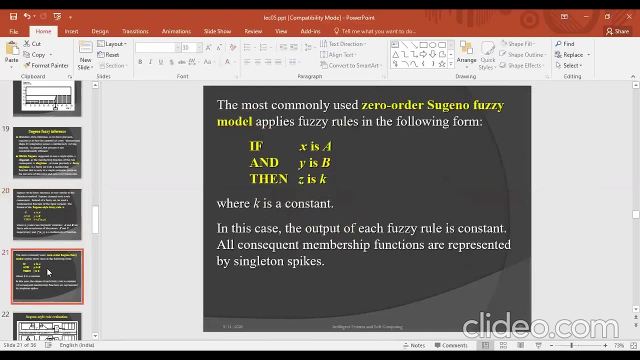 So this is the one difference between Mamdani and Sugeno: You are giving the input and in Mamdani method you are converted into membership function And here, in Sugeno method, you are converting into mathematical function. Now, the most commonly used zero order, Sugeno fuzzy model, apply fuzzy rule in the following form: 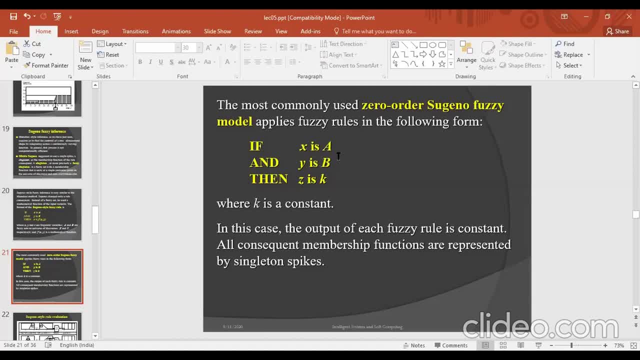 So here one rule: if x is a and y is b, Then z is k, So here k is a constant. In case the output of each fuzzy rule is a constant, All the consequent membership function are represented by a singleton spice. So you can understand this word using one example. 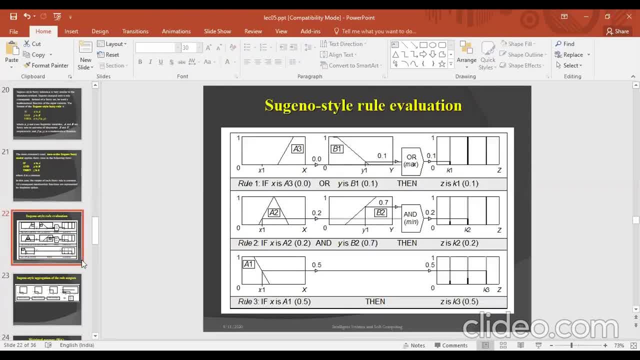 You can see here. First of all I show you the singleton style. Here I give the input rule: If x is a3, their value is zero, Or y is b1, their value is 0.1. Then the z is what is the OR operator that find the maximum of two given input. 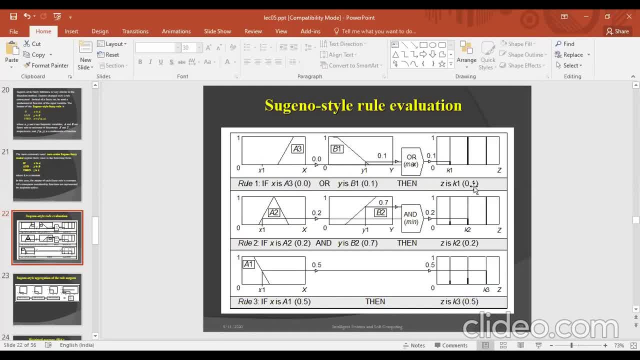 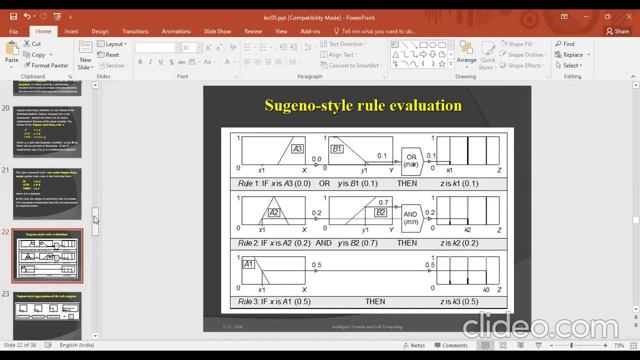 That is zero comma 0.1.. Their maximum value is 0.1.. You can see, here we are getting the only single value at your output And in Mamdani method. you can see, I show you Mamdani method. 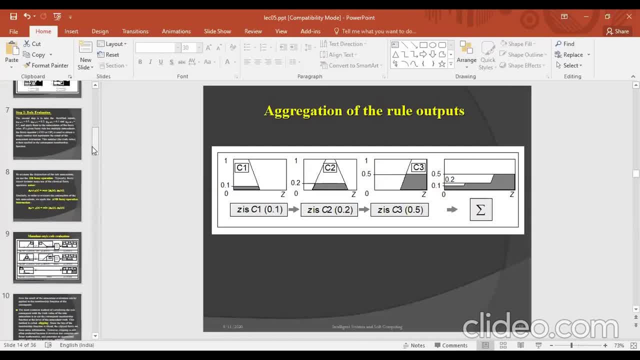 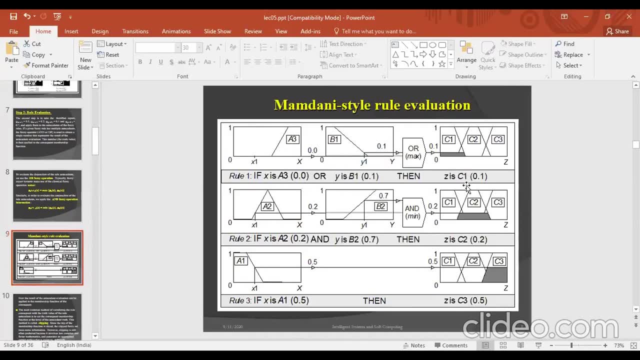 In Mamdani method you can see. You can see In Mamdani method you can see: If you are given a3, then y is b1.. Then z is c1.. The area covered by the output z is here. There is not exact or the singleton value in Mamdani method. 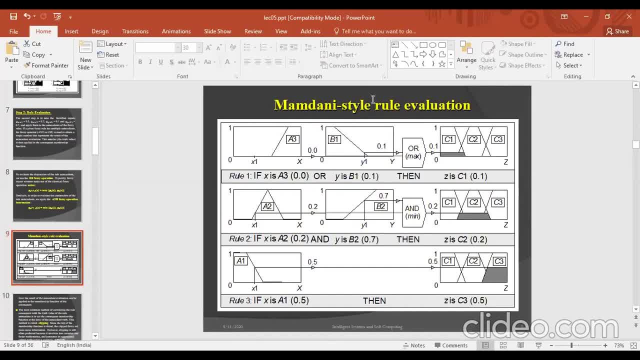 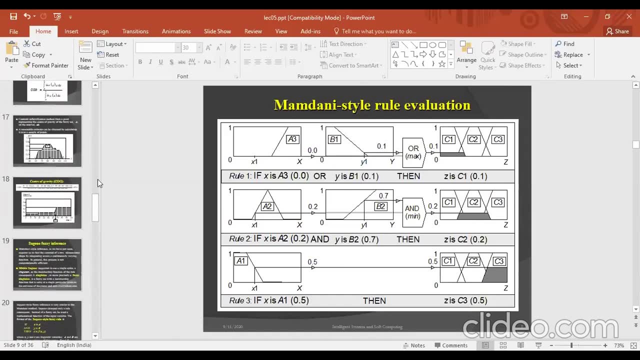 Because here we are not using the mathematical function for the calculation of your conclusion, that is z, But in Sugeno method they are using the mathematical function for calculation of your output Right? So the main difference between Mamdani and Sugeno You can see here. 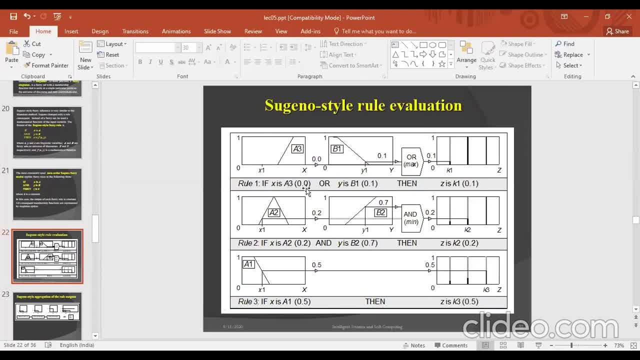 Here in Sugeno method, if you are given rule: fx is a3, their value is zero, And y is b1, their value is 0.1. Then OR operator, So OR means maximum, So then you have to find zero comma 0.1.. 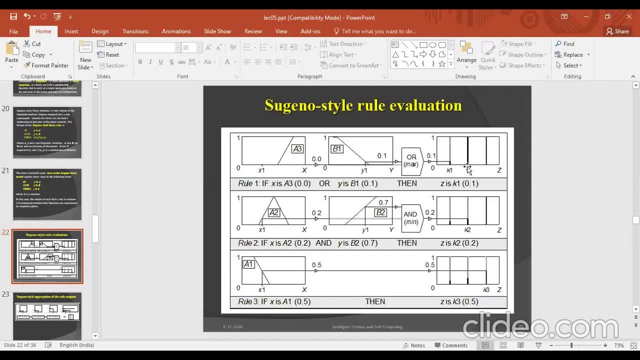 Their value is 0.1.. Here you can see the dark line. that is only singleton value. So Sugeno method: calculate your z Using mathematical function. Now, second rule: If x is a2, their value is 0.2.. And the y is b2, their value is 0.7.. 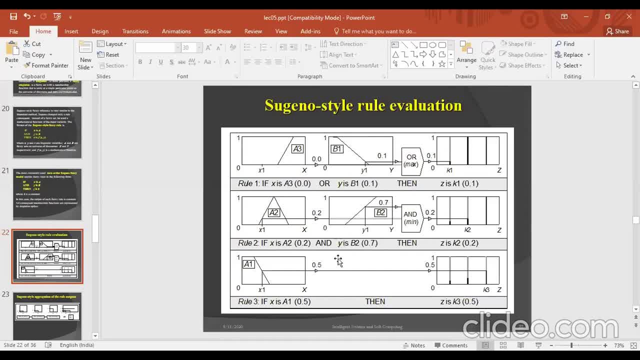 Here AND operator is used. So how you can perform AND operator? So you have to find the minimum of two. given set that 0.2 comma 0.7.. So here output is 0.2.. Okay, Now the third rule is: 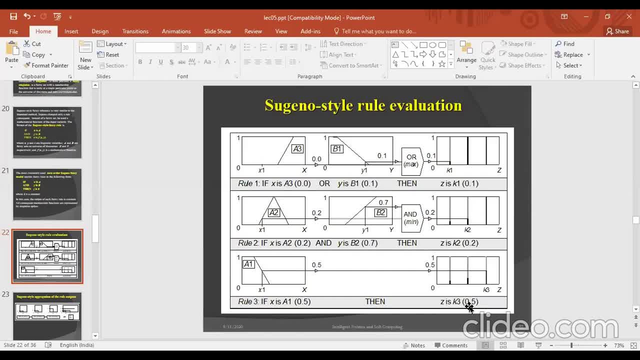 If x is a1. Then z is c1. Then z is c2.. Then z is c3. That is directly implies 0.5, then 0.5.. So you can see, Here I give x3. Then directly I calculate the output z using mathematical function. 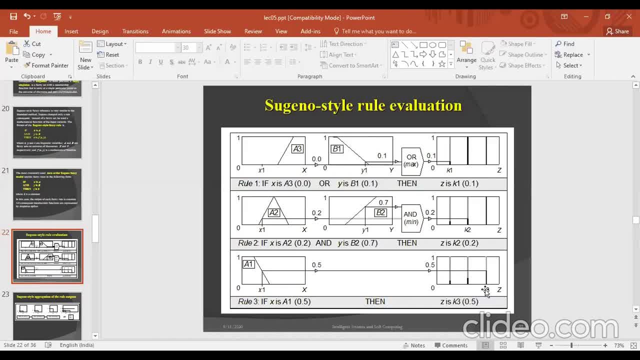 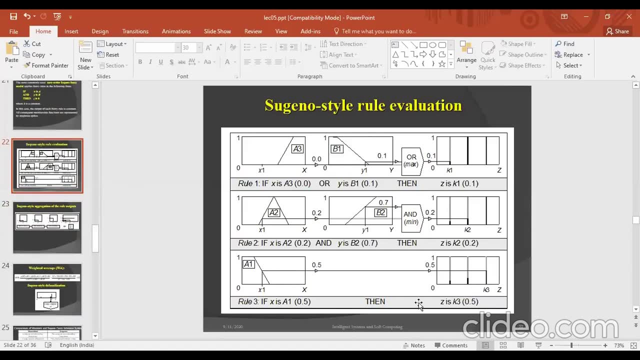 That is directly here you can see k3 point. There is no area covered between the value of the output set Only directly. you can get the singleton value of your given input Right. So why you are directly calculate This value? they use the mathematical function. 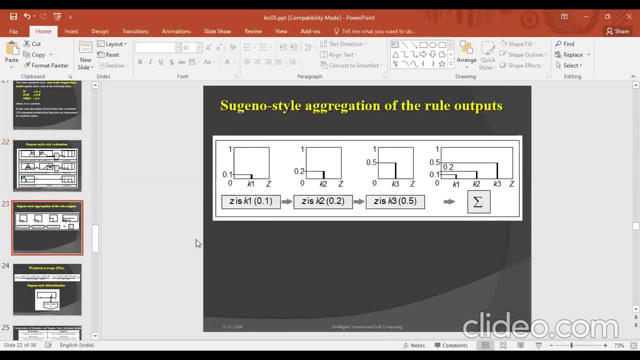 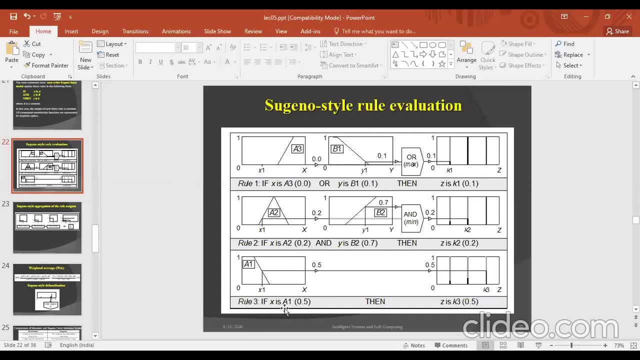 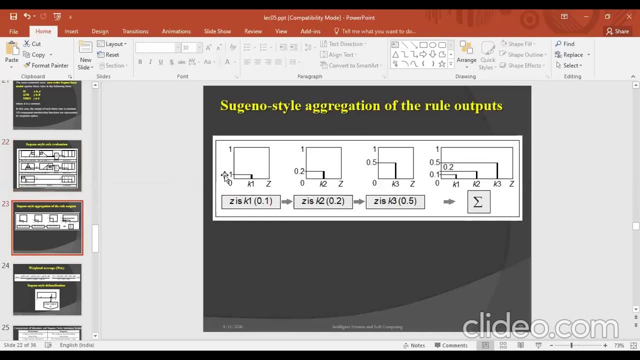 So here Now you have to aggregate the given input. Now you are applying the rule, that is, rule number one, rule number two and rule number three. So this is your output of your one, two and three rule. Right, So you can. you can see here the output of your rule one, two and three, that is k1, k2 and. 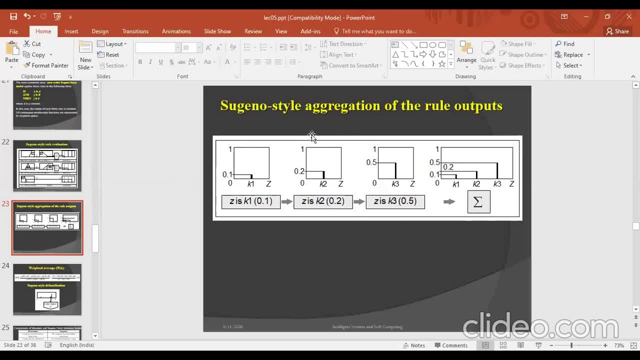 k3.. Now we have to aggregate all the output of your singleton rule. So now you have to add the input. So here you have rule. so now here k1, then k2 and k3. here the mathematical function is used to compute your. 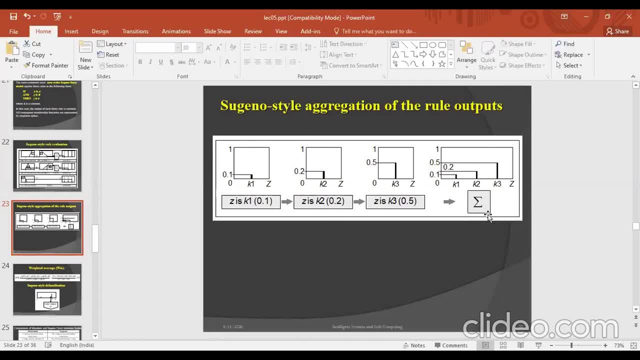 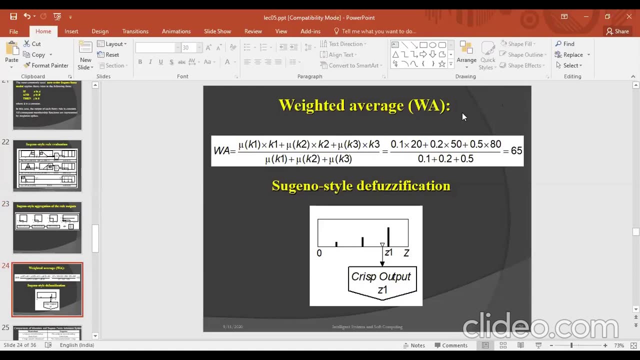 output. for last output of your system. okay, so for that, which method is used? in mamdani method we are used center of gravity method, but in single sugeno method the weighted average method is used to calculate your final output. here you can see: mu of k1 multiply a1 plus mu of k2 multiply k2. 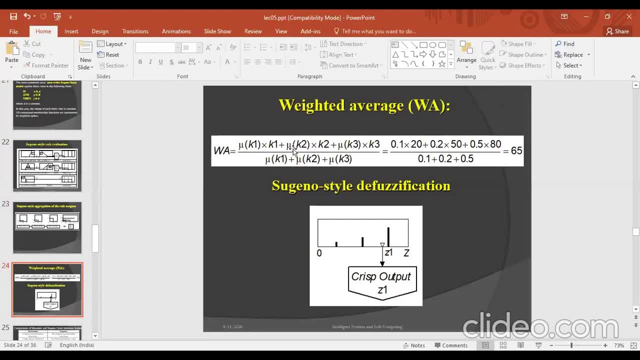 plus mu of k3, then multiply k3 divided by mu of k1 plus k2 plus k3, so you have already find the value of mu of k1, that 0.1, then 0.2 and 0.5. so what is k1, k2 and k3? that is your input, that given. 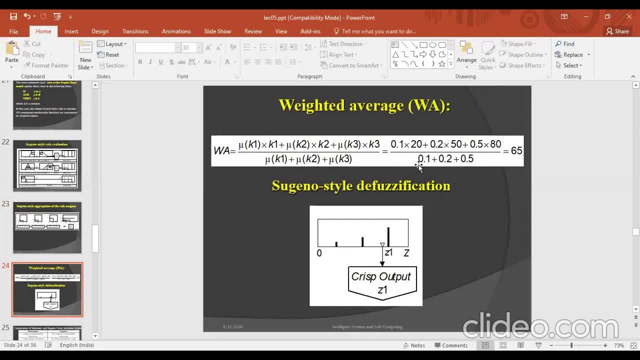 by your input. then you are divided by the mu of k1 plus k2 plus k3, the value is 65. so this is your output of your sugeno method. okay, if you have any question in sugeno method, then you can ask me a question in chat box. 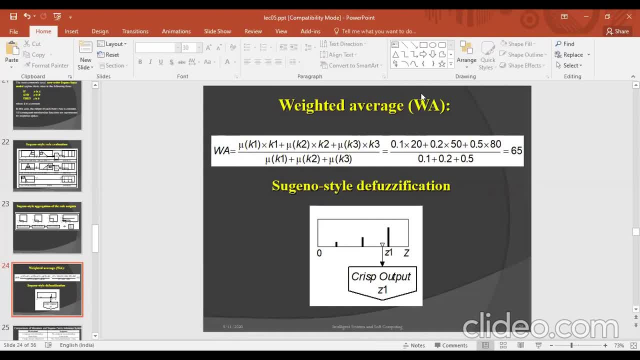 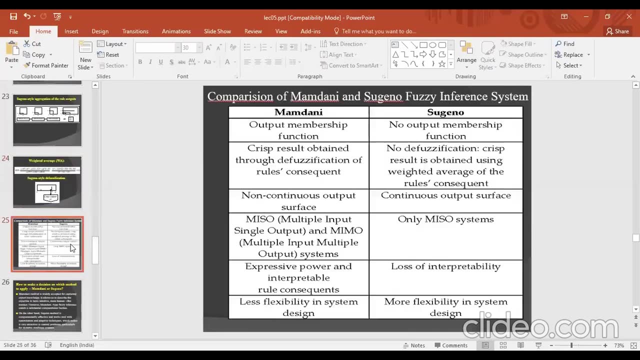 so at last we are finding or converting our method of find our input set, given input set, and then find the crisp value of your output. that is your system. so now we compare this, both the method, so you have more clear: the mamdani and sugeno method. in mamdani method we are using 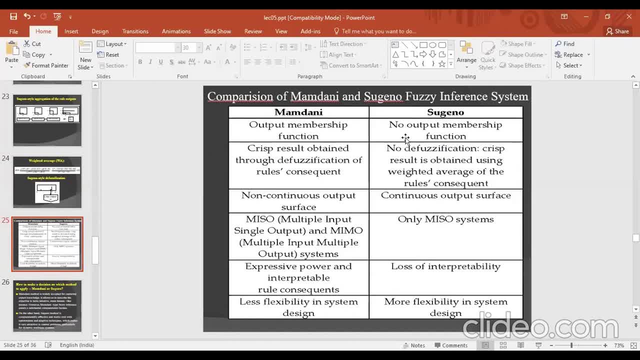 membership function and in sugeno method we are not using membership function because we are using the mathematical function. now, in mamdani method the crisp result obtained through defacification of rule consequent, but in sugeno method no disfacification required because directly we are calculating the output using this. 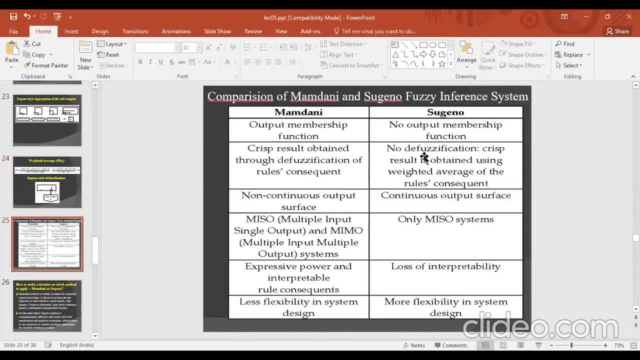 weighted average method. right, so you can see no defacification. crisp result is obtained using weighted average of the rule consequent now, third comparison is non-continuous output surface and sugeno continuous output surface. already i show you in graph format. now in mamdani method. 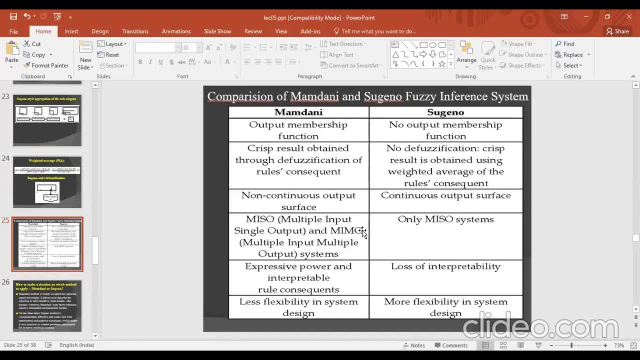 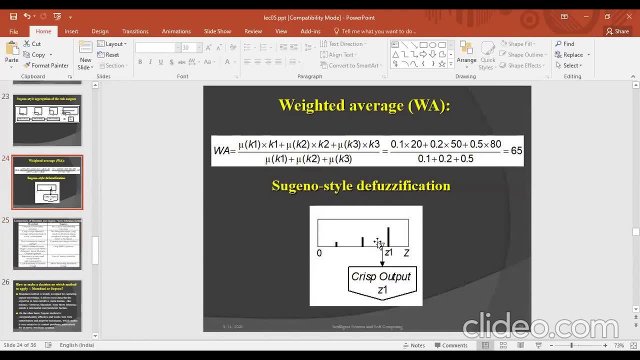 multiple input and single output and multiple input and multiple output, but only in sugeno method. only multiple input and single output is possible. you can see, here only one output is given by sugeno method. so only work for the multiple input and the single output. now third: 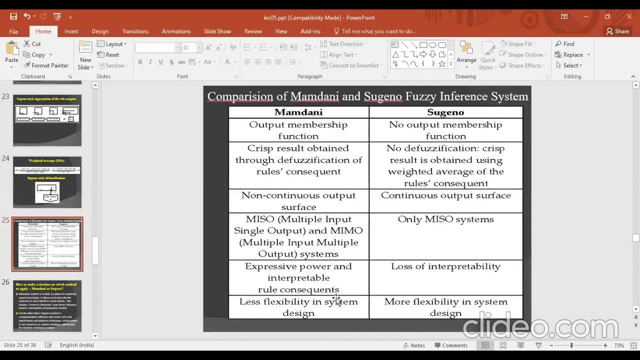 fourth comparison: expressive power and interpretable rule. consequent and the sugeno method: loss of eve interpretability. Okay Now, Mamdani method is less flexible in system design and Sugeno method is more flexible in system design. Okay, So, because we are directly use the mathematical, 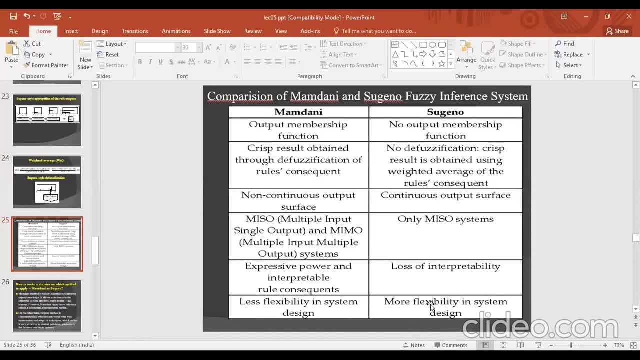 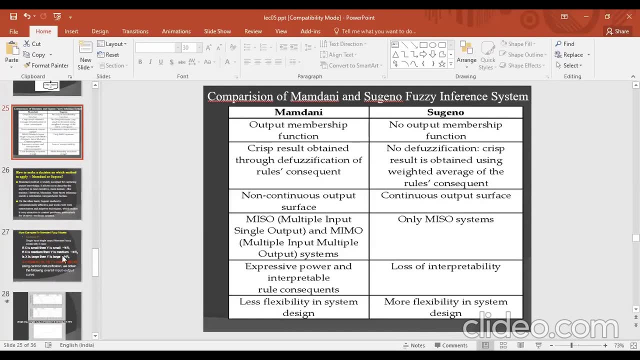 function for finalize your output. So this is a more flexible Sugeno method. Okay, I hope you have clear Mamdani and Sugeno method. If you have any question, then you can ask me a question. If you have any question, you can ask me a question in Mamdani and Sugeno method. 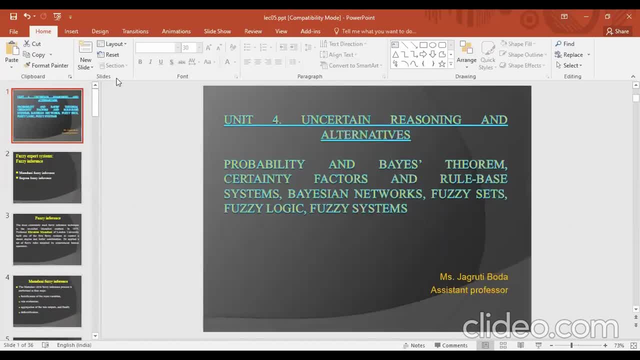 Also in your unit number four. I take the exam tomorrow at 11 to 12 o'clock. So if you have any query in probability and bias theorem, certainty factor and probability, you can ask me a question. You can ask me a question, Then you have to ready. at 11 o'clock I take the exam of unit number. 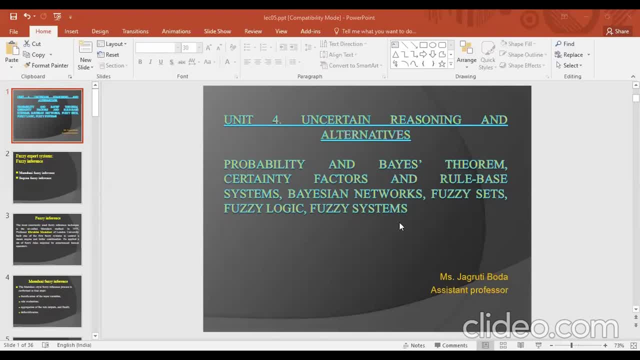 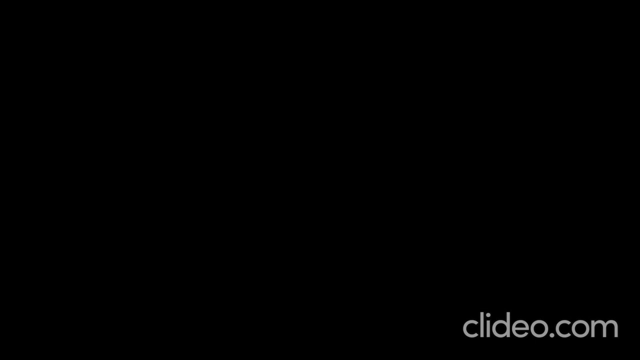 first in section two. Yes, I share my PPT in classroom today And if you require revision, then I again revise your unit number four. Yes, I worry about that, If you require revision. Yeah, okay, I devised all the concepts, so you have cleared the unit number for. 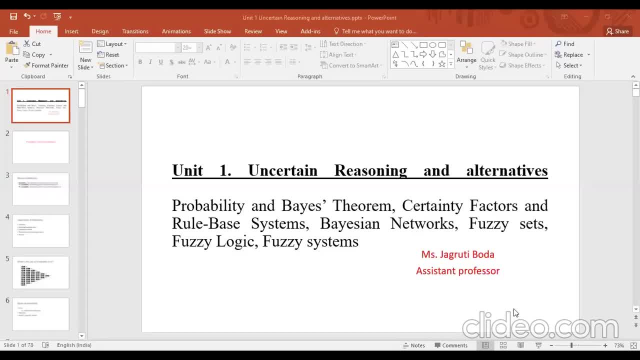 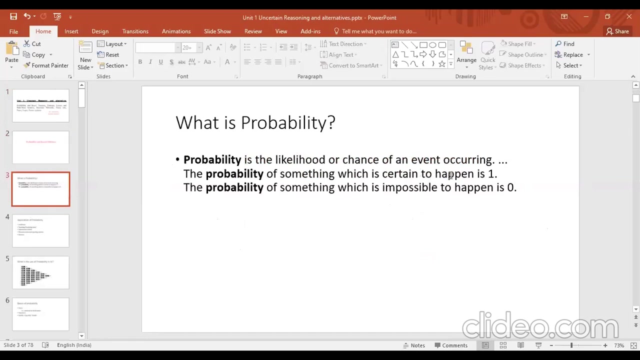 now all over the students concentrate this revision pert confrontД all the topic. so first of all is probability and bias theorem, then certainty factor, rule based system, Bayesian network and fuzzy set, fuzzy logic and fuzzy system. the first topic is probability and bias theorem. so already you know, probability is the likelihood or the chance of an event occurring, the 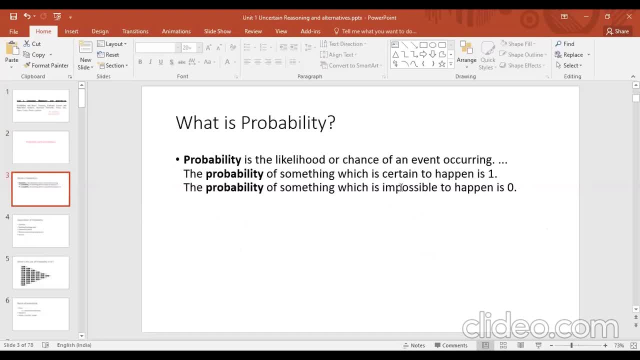 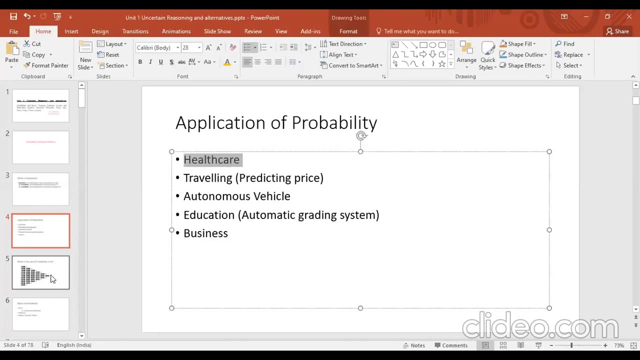 maximum value of probability is one and the impossible if there is no chance of event occurred that their value is zero. okay, so what are the application of probability? so nowadays mostly used in healthcare, traveling autonomous vehicle, education, business and all. okay, so basic of probability. you were there, these are. 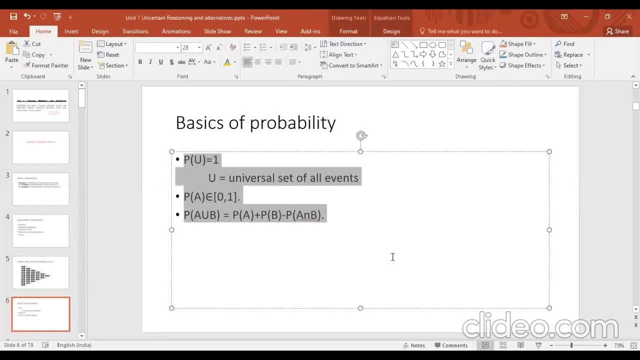 the equation that is used for the finding probability, joint probability and all probability of universal set is one and the probability of a, Z, a belongs to zero, to one, and this is the formula for finding the probability of a union B, that is, probability of a plus B. 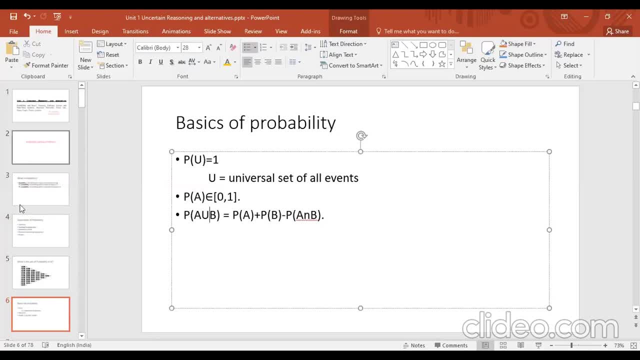 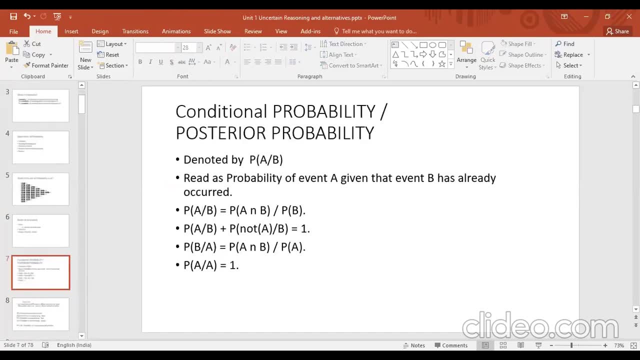 minus a intersection B. okay, now conditional probability. so what is conditional probability? we means probability of a over B. means you already the B event is occur and then the event a is occur. this is called as a conditional probability, or post shared probability, to probability of a intersection b divided by probability of b. okay, uh, now example. already we 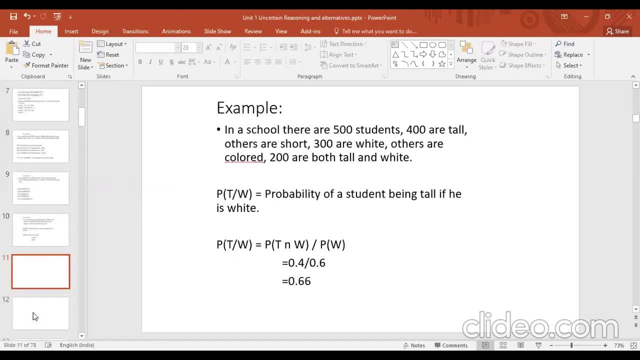 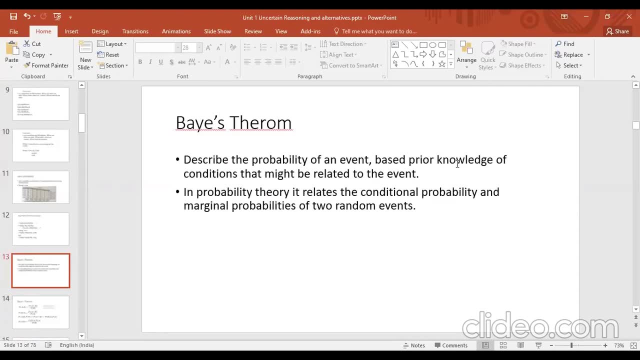 have uh calculate this example. so i directly comes to the main topic, that is, bias theorem. so describe the probability of an event based on the priority knowledge of condition that might be related to the event. so suppose you are the uh told the example of feather prediction. so we are using the previous data or the previous weather data, and then, based on that data, we are 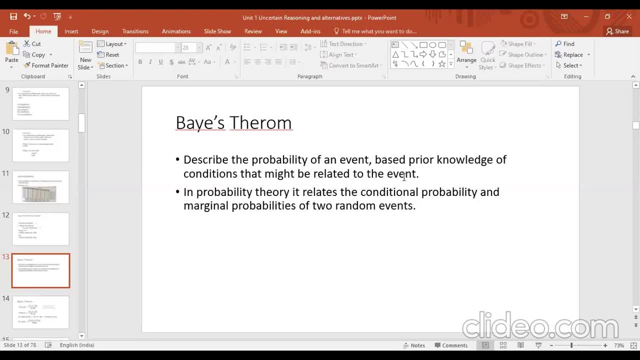 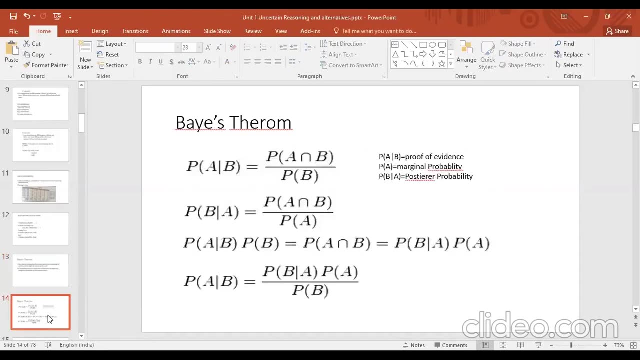 find the probability of rain is occur or not. predict the weather. so this is mostly based on your, based on your probability theory. so bias theorem is based on the probability theory. you have to find conditional and the marginal probability of two random event. and what is the formula for bias theorem? so probability of a. 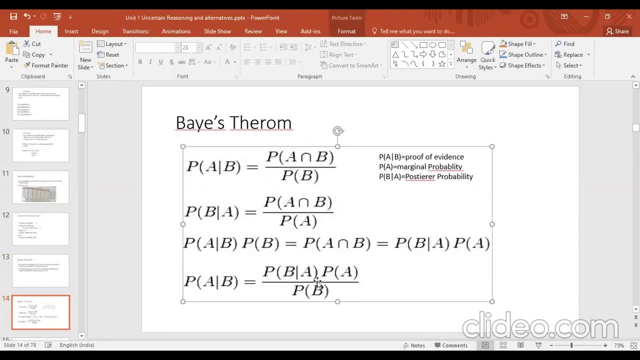 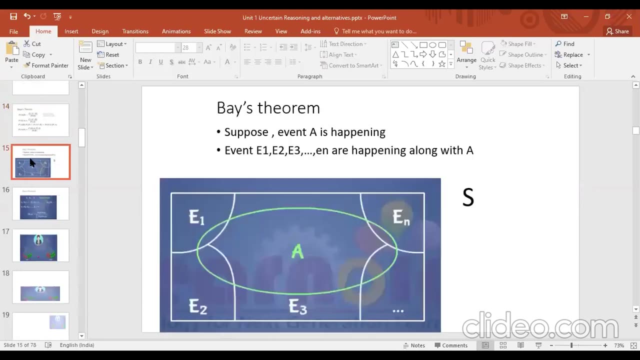 over b is equal to probability of b over a, into probability of a divided by probability of b. so you have remember this formula, the bias theorem, formula for calculation of conditional probability. now, already we have solved this example. if you have two bags and you have to drone a, one, red, 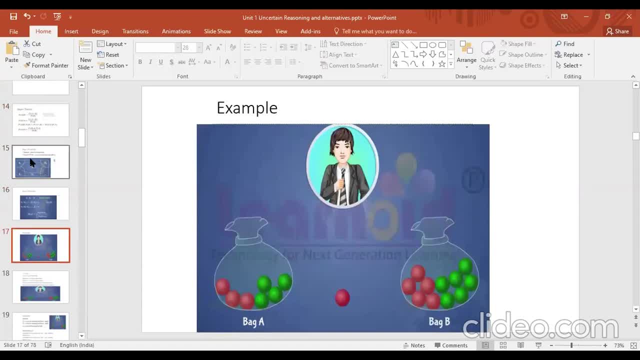 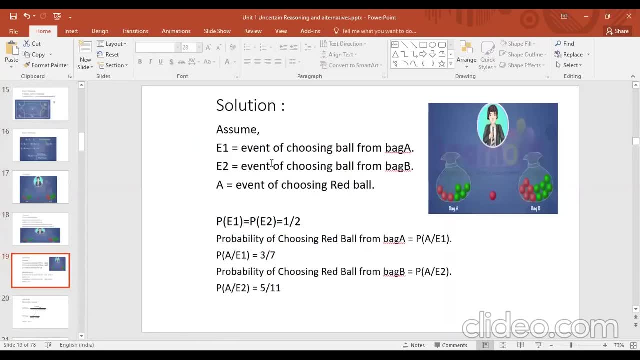 ball from your bag b. so what are the possibility? first of all, you can select from any of the bag, so you can easily change the exact number of a 2 one to the one. so now my first step is to calculate the probability of a letter b, an event. 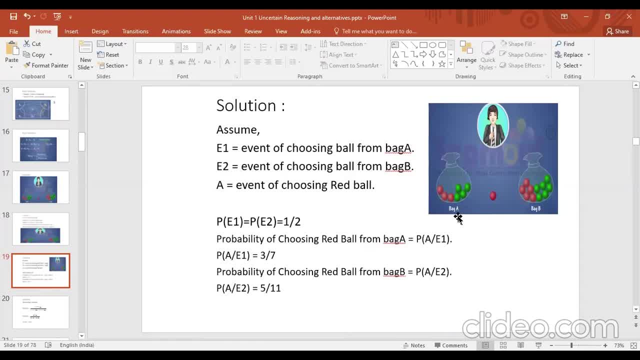 because here is loom. we are looking to evaluate which end between bag a and e1, cell a's shall. what is the probability that when e1 and event, e1 and e2 event, suppose you are selecting from bag a, then what is the probability? so one upon two? because you have a two bags and what are the chances of you are drawn the red ball from bag a? so in red block red bag you have a 3 red ball, so 3 upon 7, so total ball are in bag a are 7, so 3 upon 7and in b, so 5 upon 11un. yes, possible, so i have let you know here. 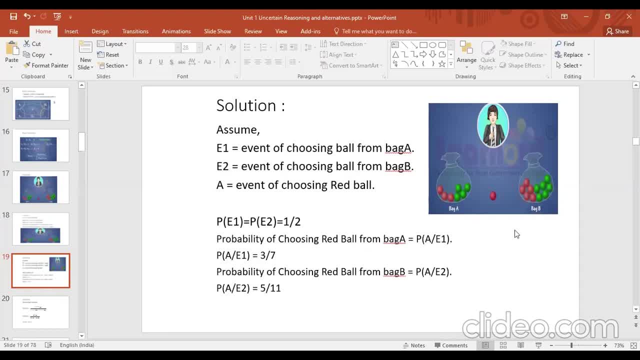 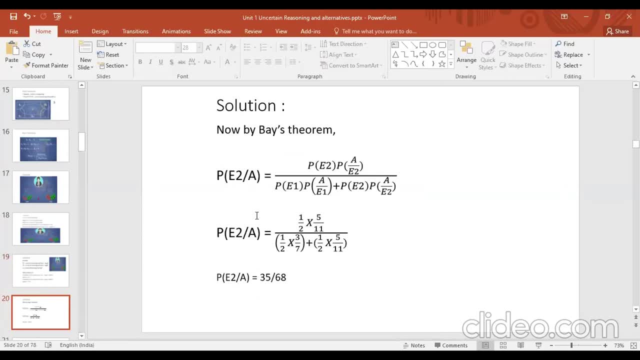 red ball, red B, you have a five red ball and total number of polar: 11.. Now you have to find the probability using Bayer's theorem. So you have to draw on a red ball from red B, So E2 over A. So you can use this Bayer's formula and calculate the output of your problem. 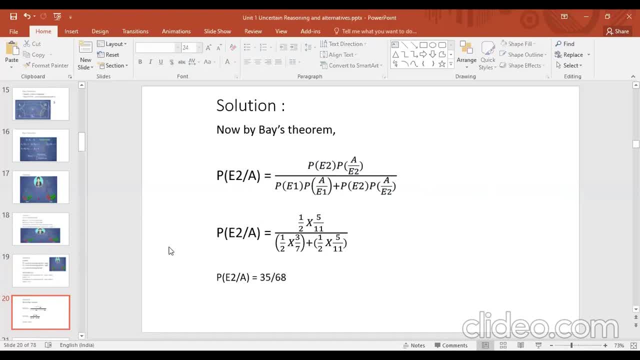 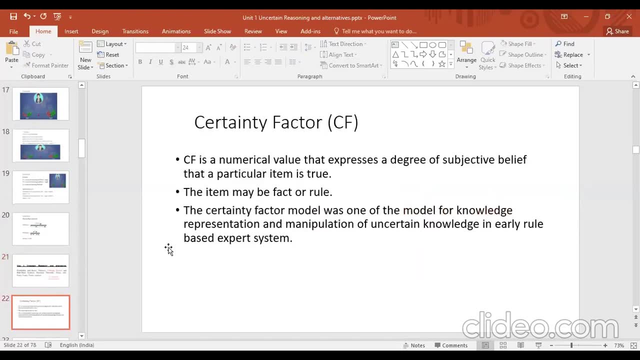 Okay Now what is certainty factor? Sometimes you have not given the probability value to solve your problem, So what you have to do, So CF is a numeric value that express the degree of subjective belief that a particular item is true. The item may be fact or the. 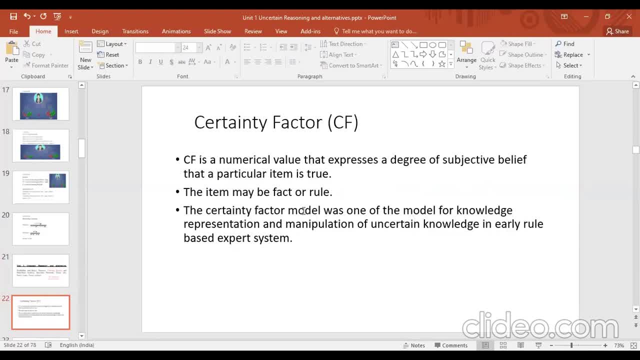 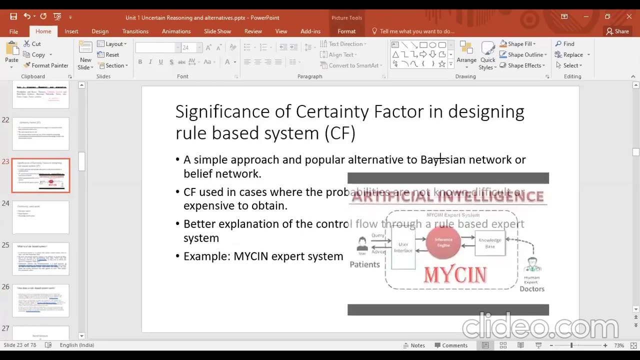 rule. So certainty model was one of the model for knowledge representation and manipulation of uncertain knowledge in early rule-based system. So before, if you have not a value of given input- that is, probability- then you can use certainty factor. The most popular AI system is your. my scene, So my scene is your, you. 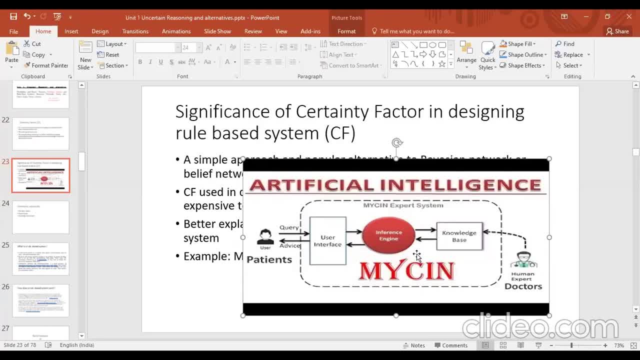 have to search on Google. What is my scene? So if this is based on the expert system relating, you have to find the uh uh advice from your uh any disease. So user directly uh interact with the system using interface like mobile or web application. 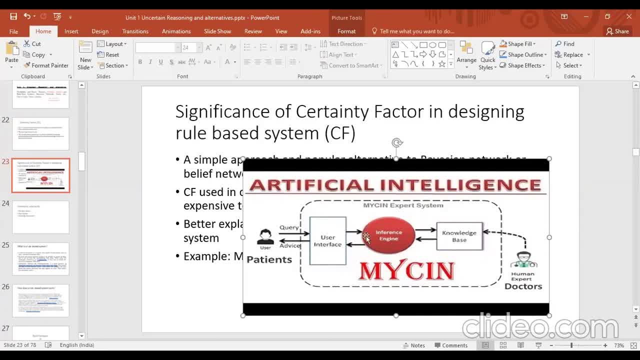 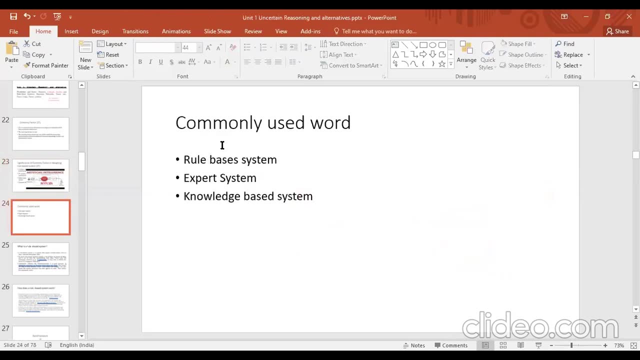 And the interface engine process the query of your user and the knowledge base consent the all the human, expert doctor knowledge. So you uh, their, their knowledge is written in the knowledge base. Okay, So this is your simple rule-based system. So, uh, you can. 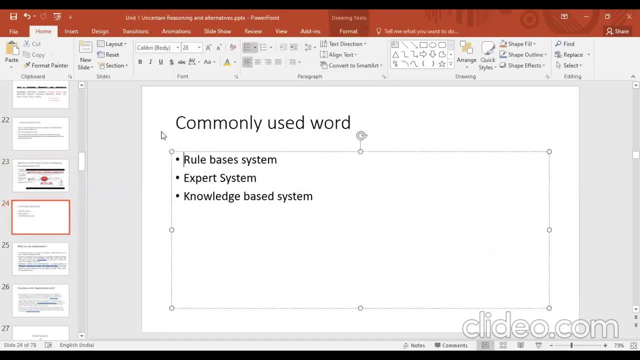 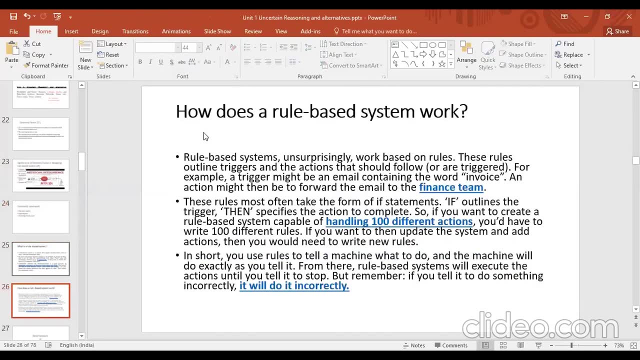 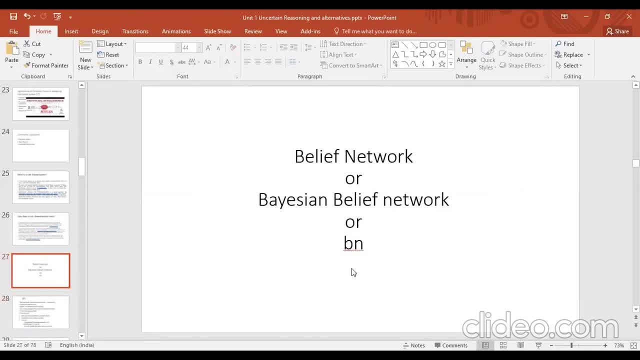 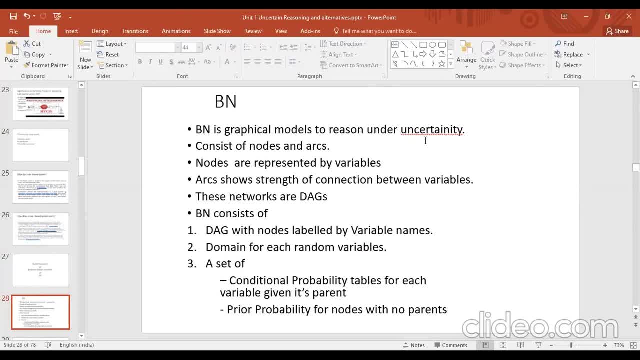 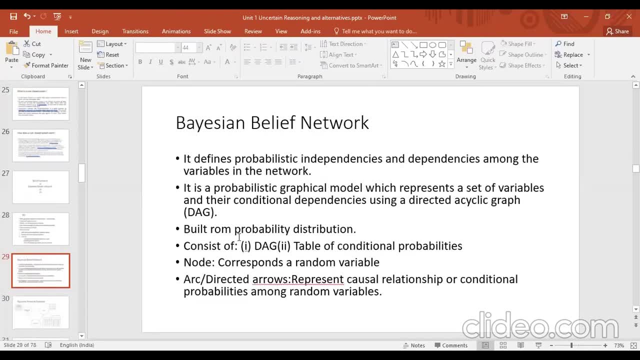 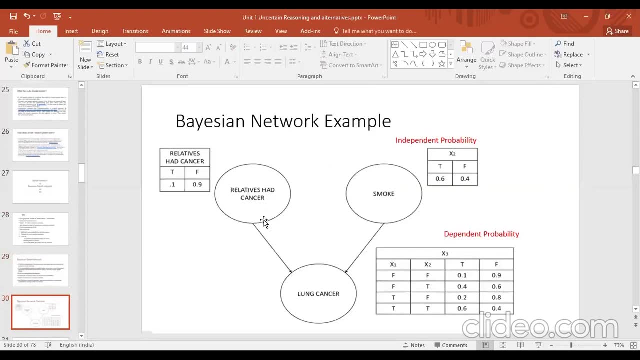 This is a graphical model to reason under uncertainty. that contain the DAG means directed acyclic graph and the probability table. So you can see here this is your sample Bayesian network- that contain nodes and arc. So DAG, contain the nodes and arc. What is DAG Directed? 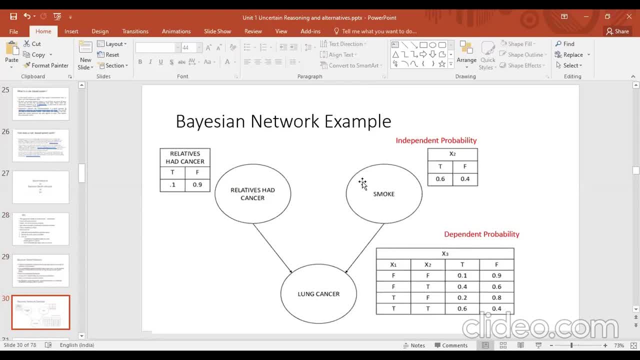 acyclic graph: node connected with each other, but they are not making a cycle. If relative head cancer directly link with the smoke, then they make a cycle. So this is not your directed acyclic graph. okay, So here you can see. Bayesian network contain nodes and arcs. 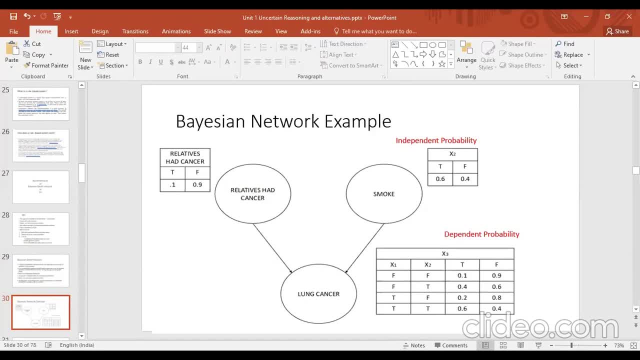 and the node arcs are linked with the two node and that contain the probability table. Here you can see relative head cancer and the independent probability table. And here you can see lung cancer is dependent on these two events, right? So there is the dependent probability table. 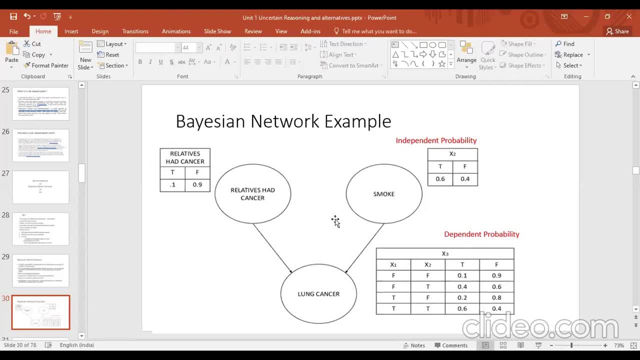 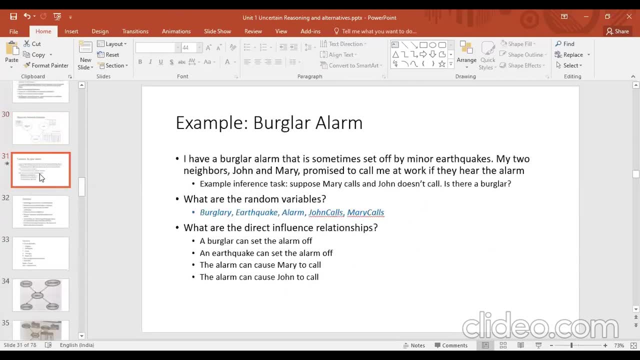 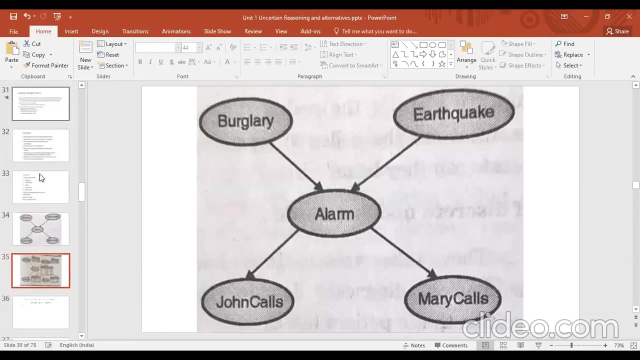 If the chances are true, both are true, both are false and one is true. so you can see here the Bayesian network example. Okay, so you can already have implemented this practical Already. we have covered this Burgundy-Alarm example in Bayesian network. 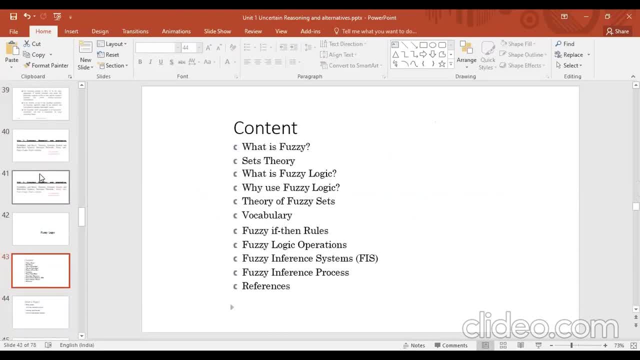 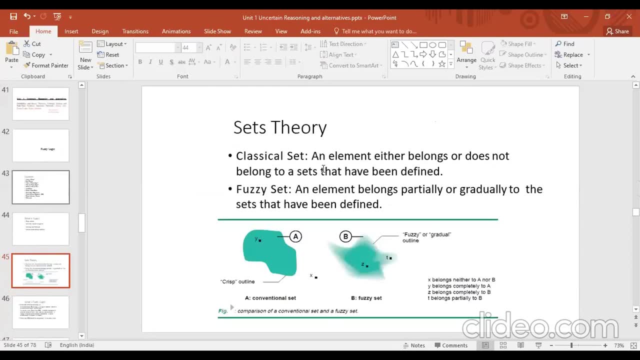 Now the next topic is fuzzy set. So what is fuzzy? So fuzzy means not clear, not crisp or the blur Means that have not exact value. Suppose you are giving the temperature 25 degree, So this is your crisp value or classical set. 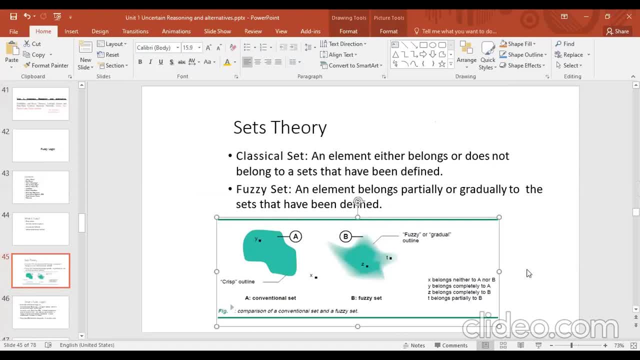 But fuzzy set, you can say the temperature is cold, hot or a very normal condition. So these are the word fuzzy set. So how you can? the system can understand. So that's why we require fuzzy set. So it has a two different meaning. 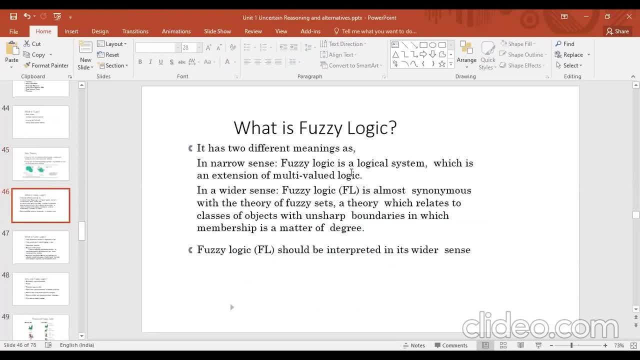 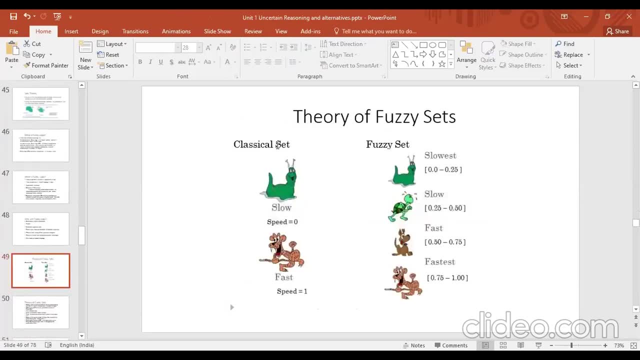 Fuzzy logic is a logical system which is an extension of multi-value logic. Okay, so here I give one example. You can see here, so classical: set the speed of your bike. that is slow and fast You can take value. speed is equal to zero. 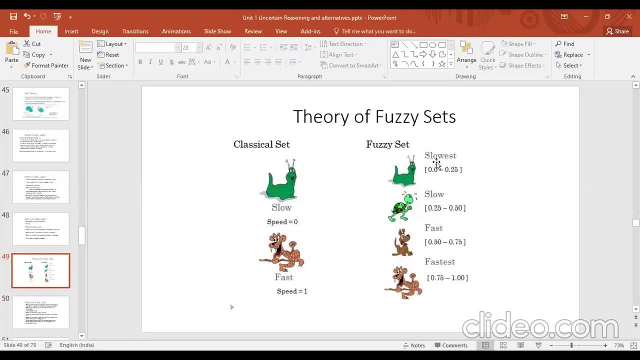 and speed is equal to one. Suppose you have multiple value, this slowest, slow, fast and fastest. So you have to. given the value of your slowest speed, that is zero to 0.25, then 0.25 to 50,. 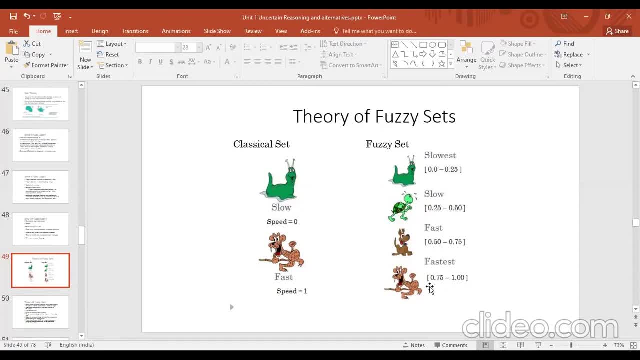 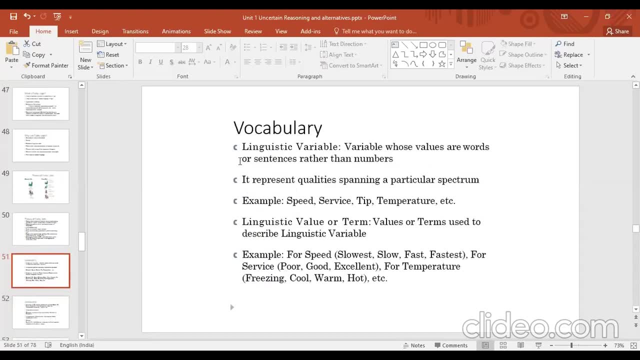 then 0.50 to 0.75 and 0.75 to one. Okay, so you have to require a fuzzy set for a linguistic variable. What is linguistic variable? The variable whose value are words or sentence rather than the number.